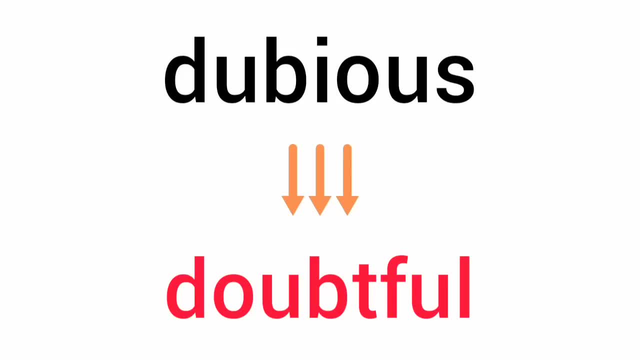 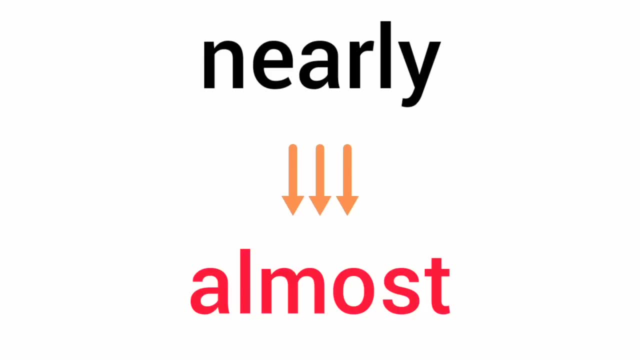 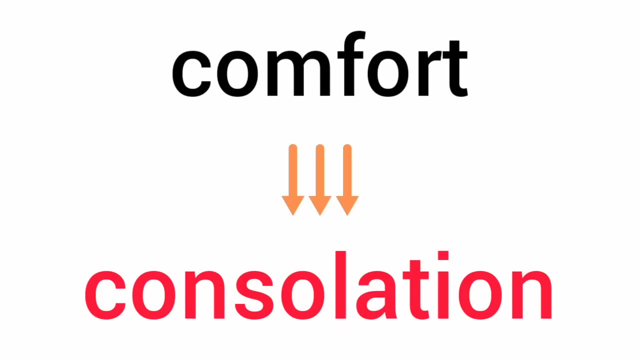 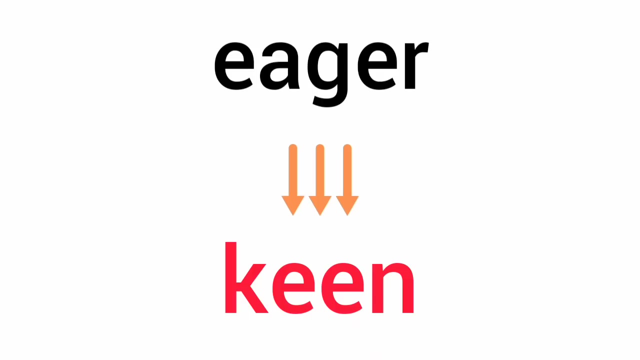 dubious, doubtful, Nearly, almost, nearly almost. Comfort, consolation, comfort, consolation, Eager keen, eager keen. Nearly, nearly, nearly, nearly, Near, close, near close, Lively animated, lively animated. 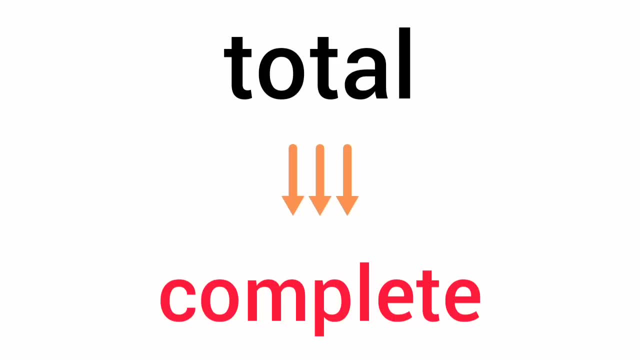 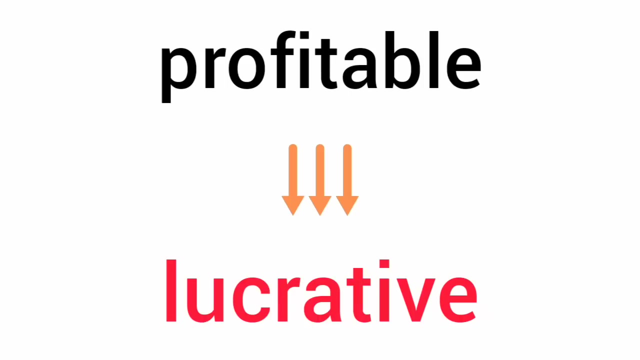 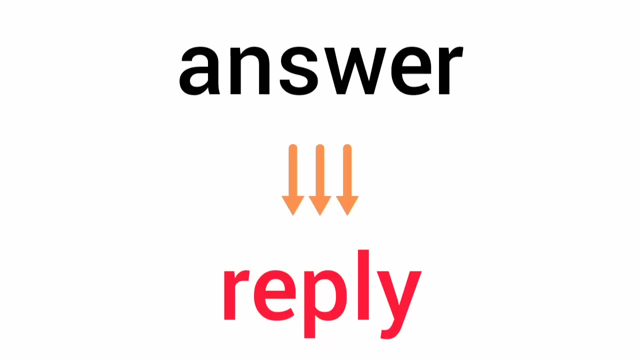 Total, complete, total, complete Earth soil, Annoy, irritate, annoy irritate. Peace, harmony, peace. harmony, Profitable, lucrative, profitable. Anser reply. user reply. Confine restrict, confined restrict. 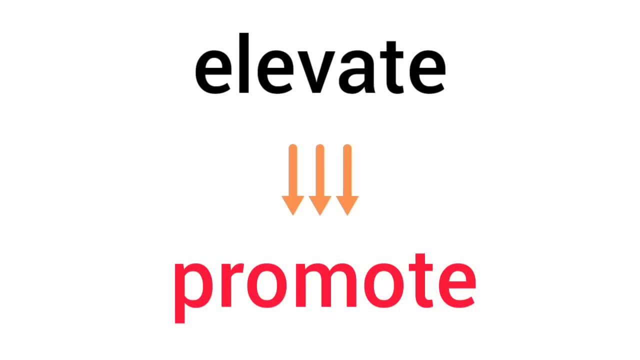 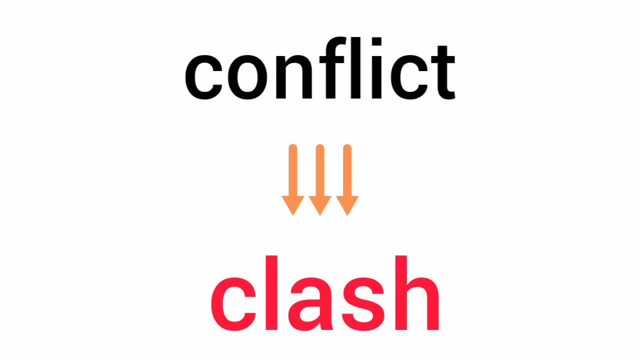 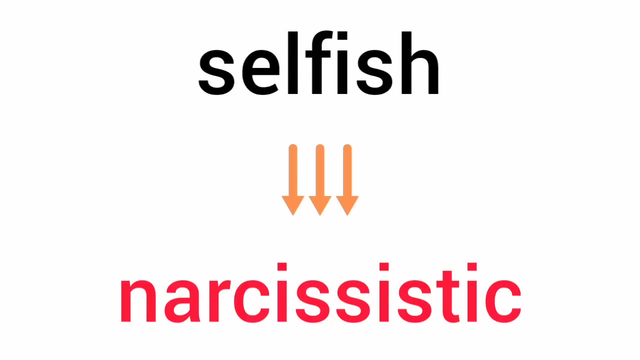 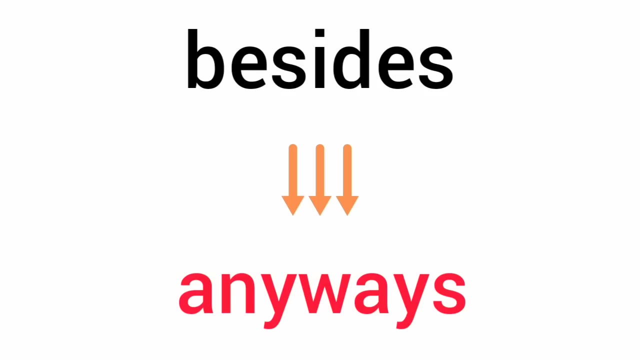 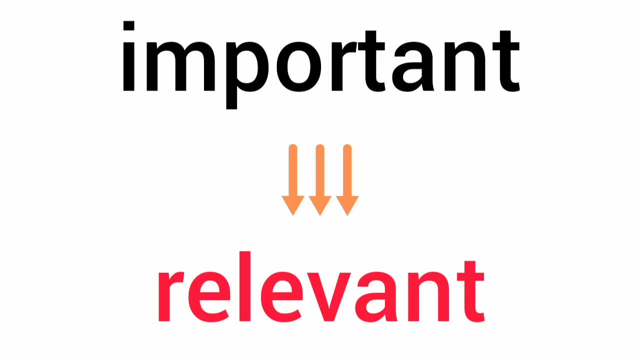 Elevate, promote, elevate, promote, Elegate, promote My fortune, My fortune, Conflict clash, conflict clash, Selfish narcissistic, selfish narcissistic, Besides, anyways, besides, anyways, Important, relevant, important, relevant. 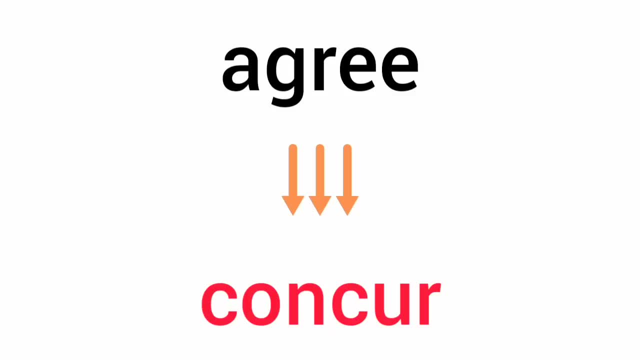 Agree, concur, agree, concur, Submit, comply, submit, comply, Stress, Emphasize, stress, emphasize, Connect, join, connect, join, Friend, ally, friend, ally. Huge, enormous, Huge, enormous. 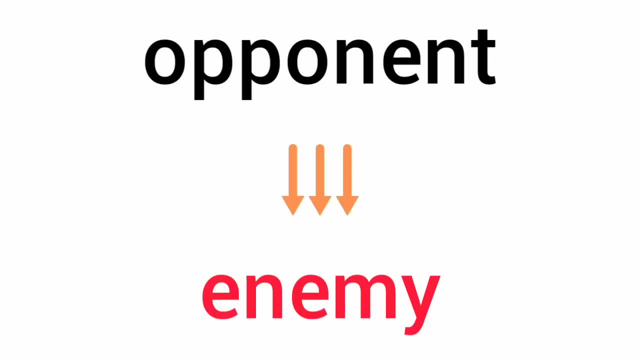 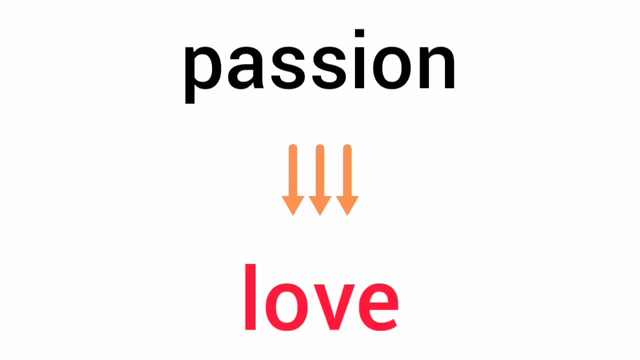 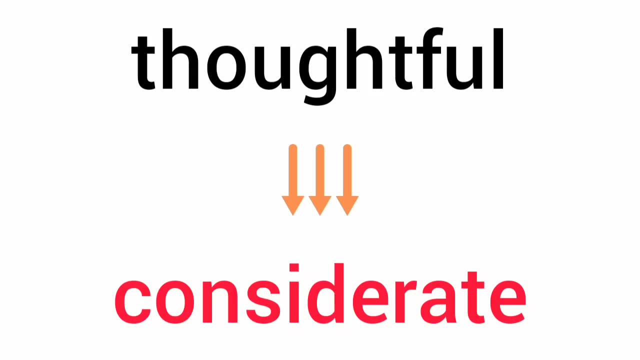 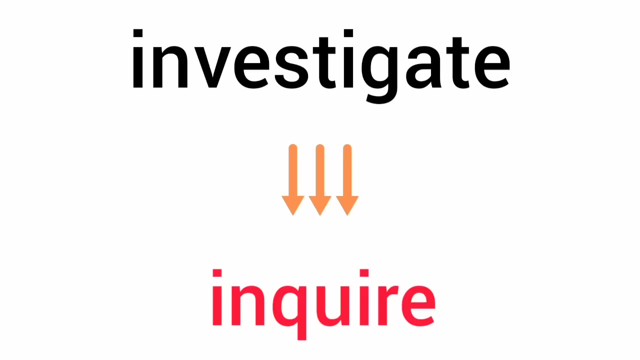 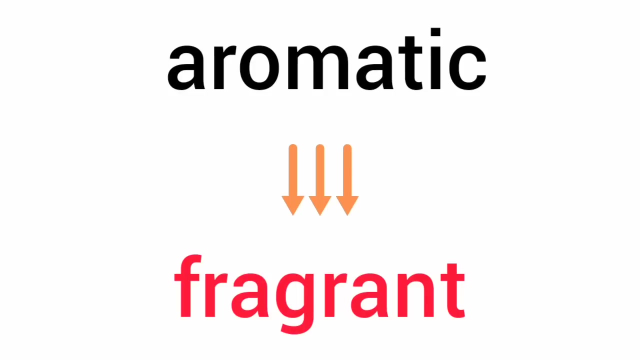 Opponent, enemy, opponent, enemy. Passion, love, passion, love. Thoughtful, considerate, thoughtful, considerate, Considerate, Investigate, inquire, investigate, inquire. Aromatic fragrant. aromatic fragrant. 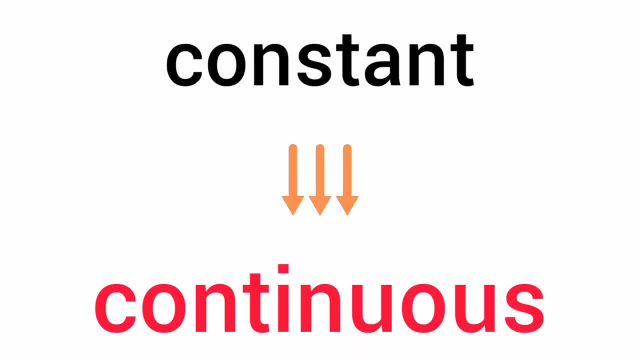 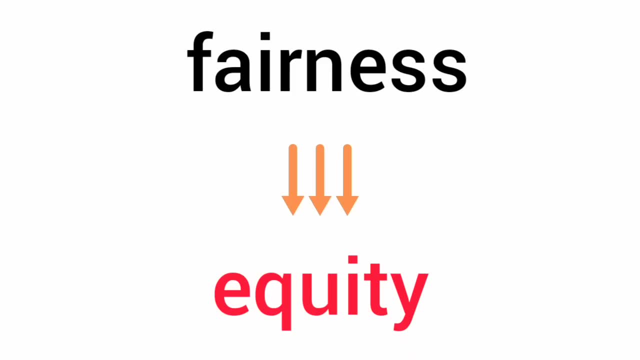 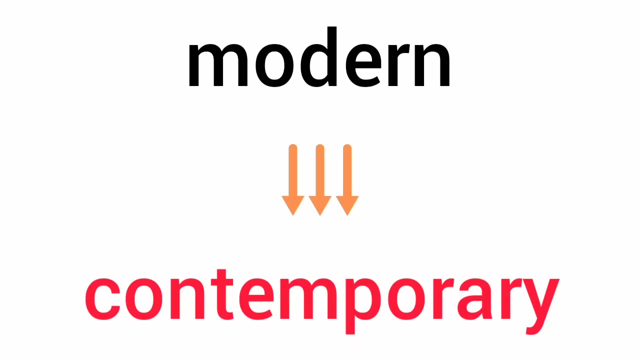 Constant, continuous, constant, continuous Submit Fairness equity, Fairness equity, Fairness equity. Reach arrive, Reach arrive. Modern contemporary, Modern contemporary, Especially modern, contemporary, Especially successful. 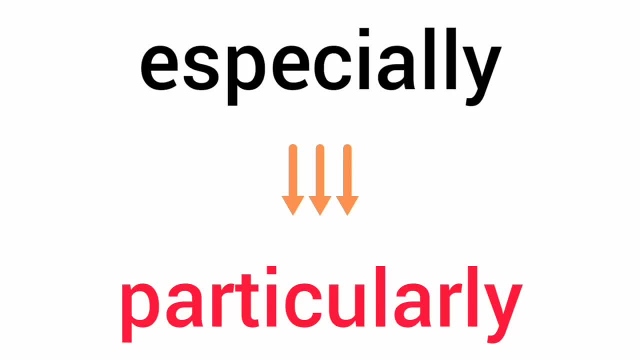 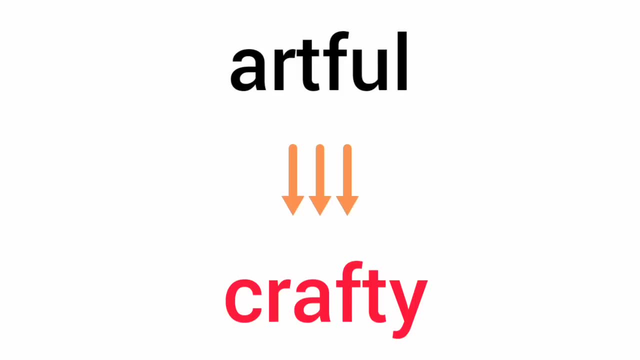 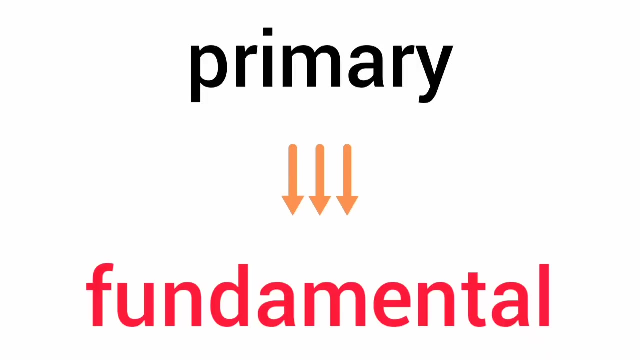 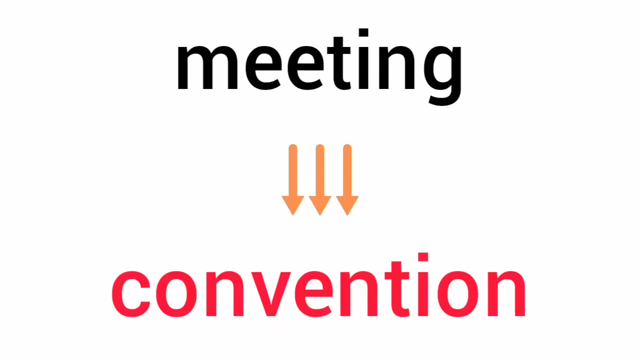 nome next: washinurcom: Watch, Watch, Watch, Watch, Watch, Watch, Watch, particularly especially particularly artful crafty. artful crafty. opposite, contrary opposite, contrary primary, fundamental primary, fundamental meeting convention. 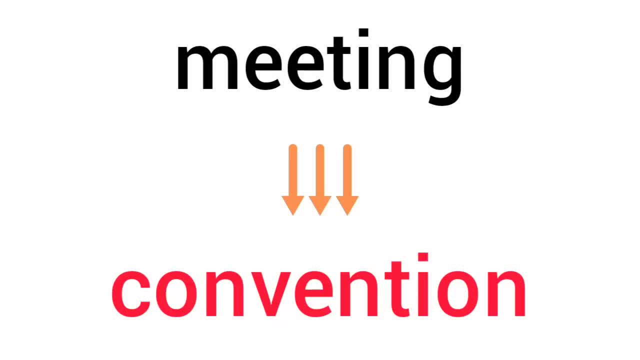 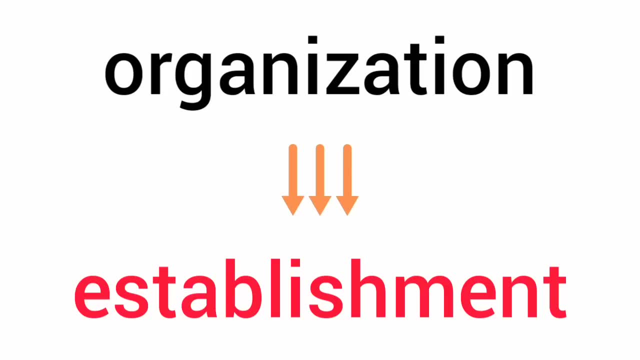 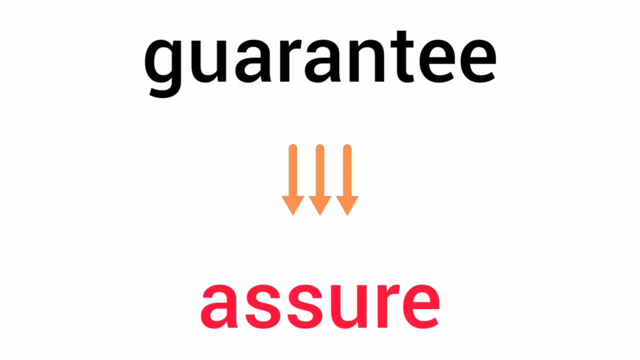 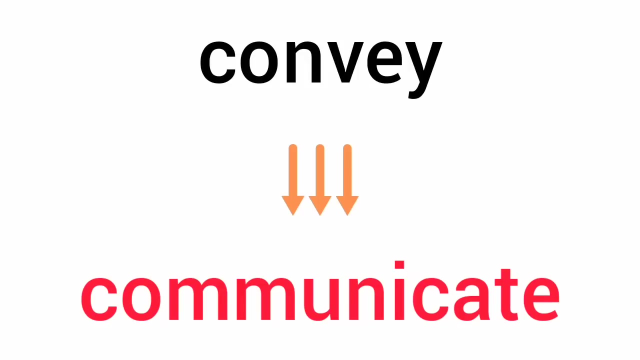 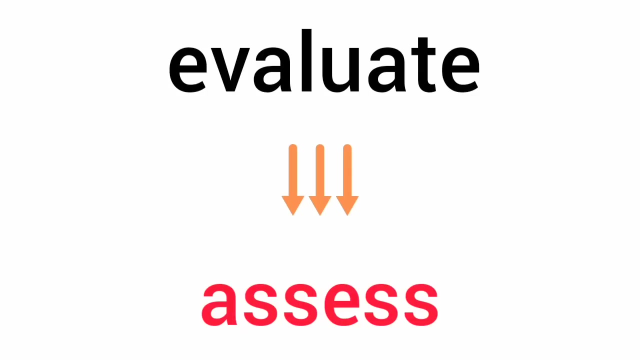 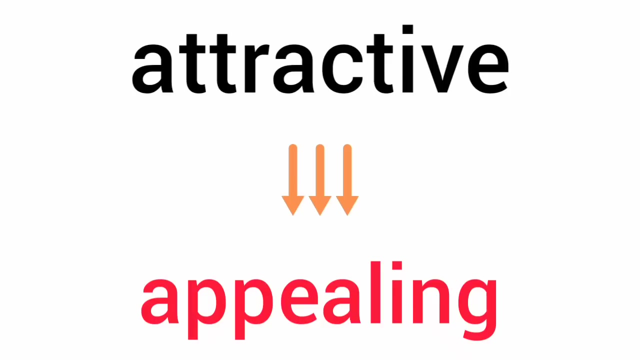 meeting: convention: organization establishment, organization, establishment, guarantee, assure, guarantee, assure, convey, communicate, convey, communicate, evaluate, access, evaluate, mitigate number, number, measure number. Taylor suggest: subtract, repeat, be, be to going. 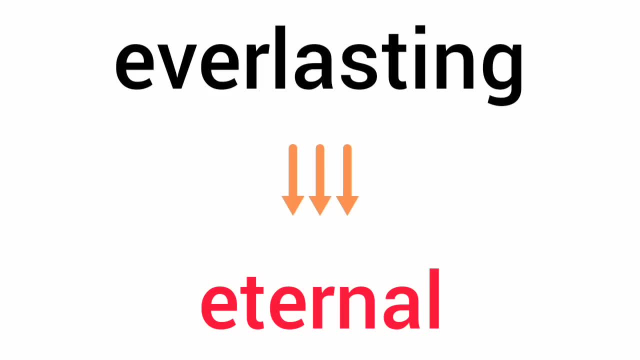 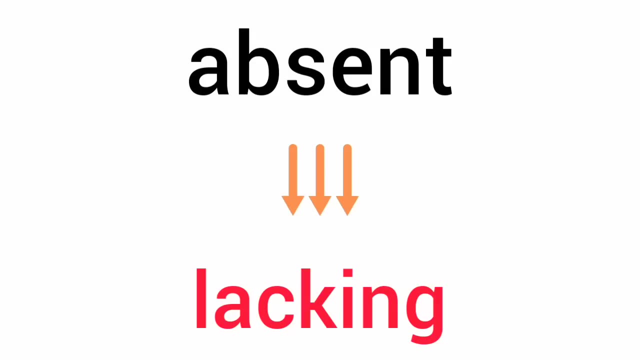 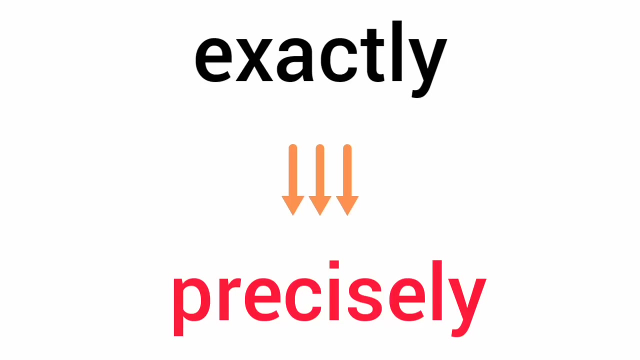 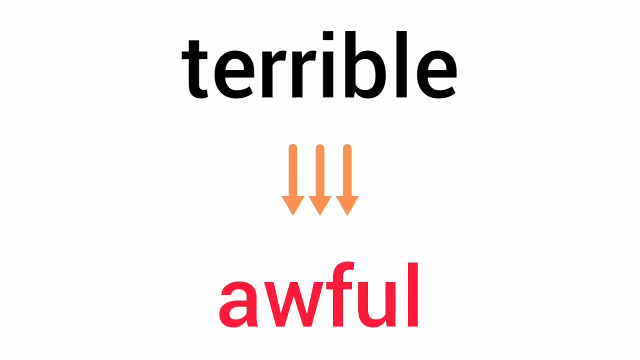 hold encouraging laufen, such 80, attractive appeal, attractive, appealing, attractive, appealing, manage, cope, manage, cope, everlasting eternal, everlasting eternal, absent, lacking, absent, lacking. right, correct, right, correct, exactly, precisely, exactly, precisely. 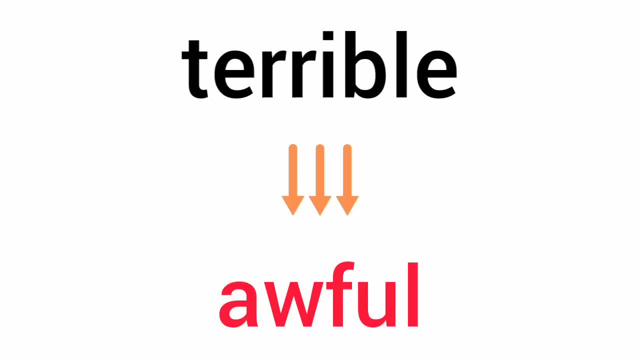 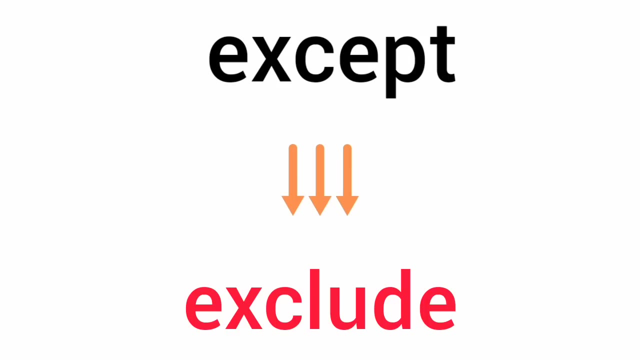 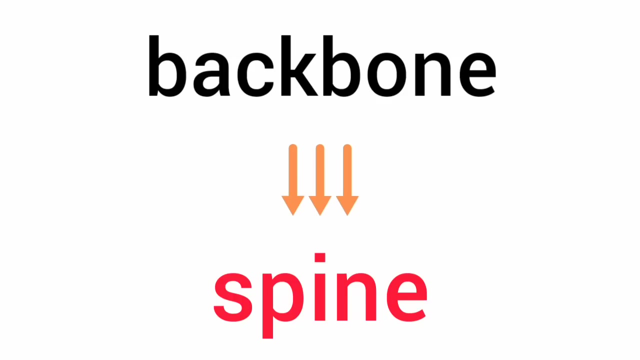 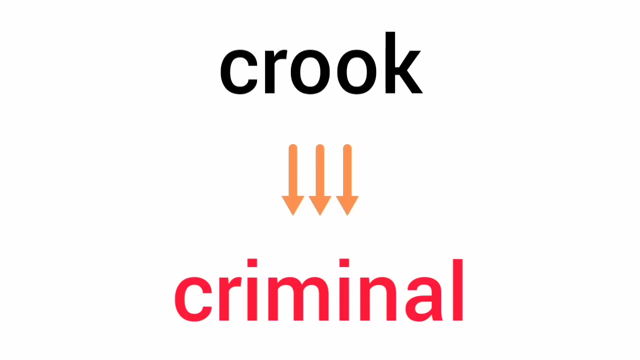 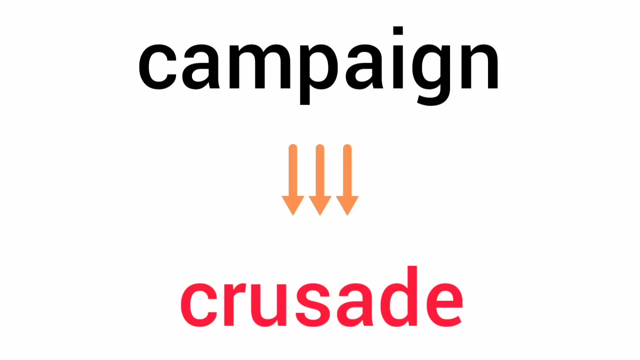 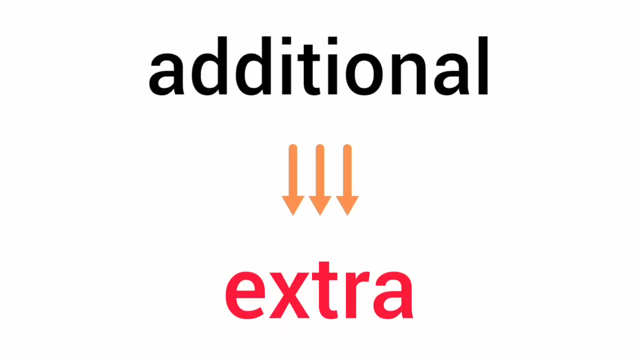 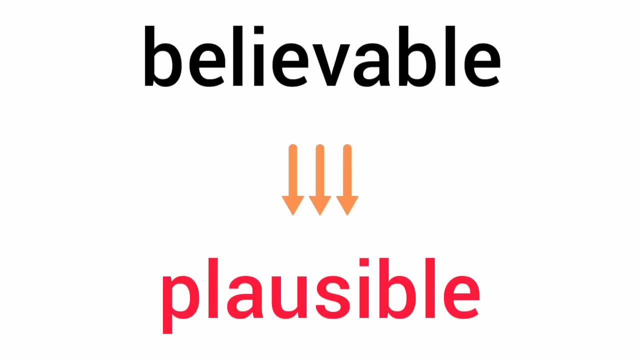 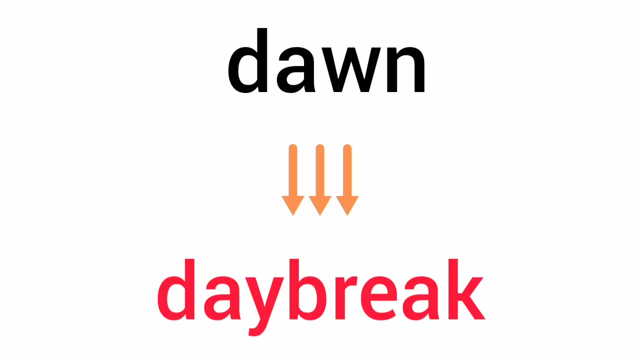 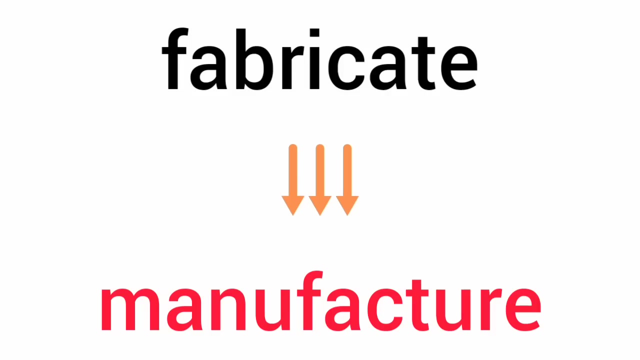 terrible, awful, terrible, awful couch sofa, couch sofa, except exclude, except exclude, backbone, spine, backbone, spine, crook, criminal, crook, criminal, explode, blow up, explode, blow up, start, begin, start, start, begin, campaign, campaign, crusade, campaign, crusade, additional, extra, additional, extra, believable, plausible, believable, plausible, Dawn, daybreak, dawn, daybreak, fabricate manufacture, fabricate manufacture. 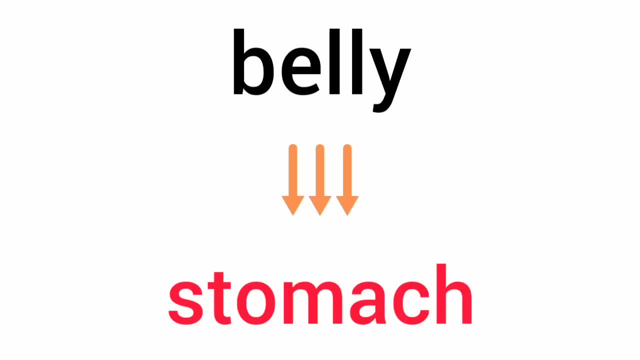 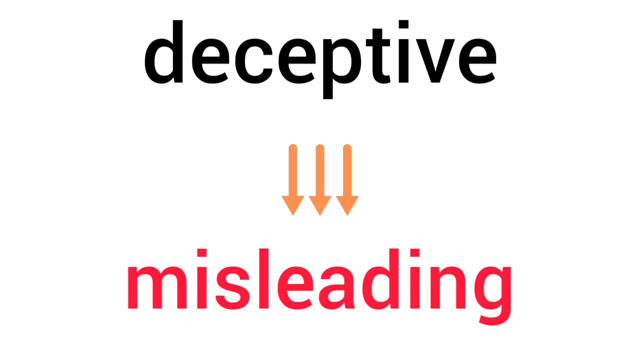 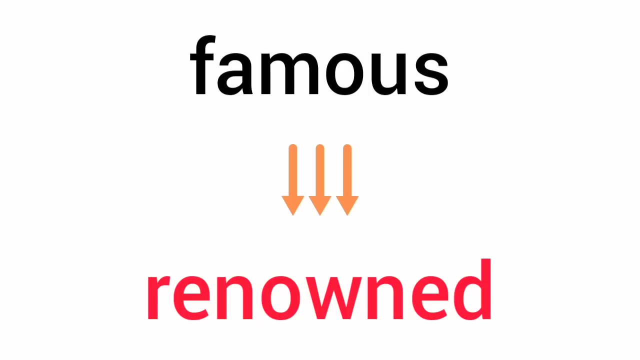 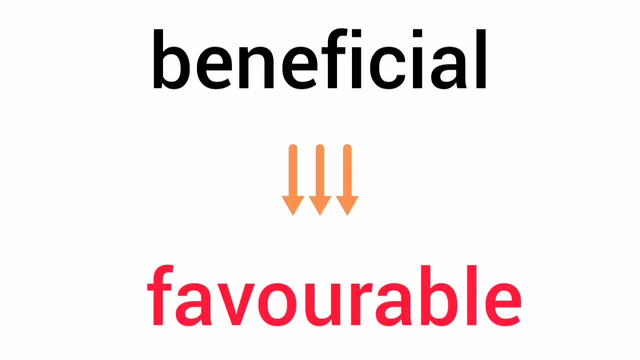 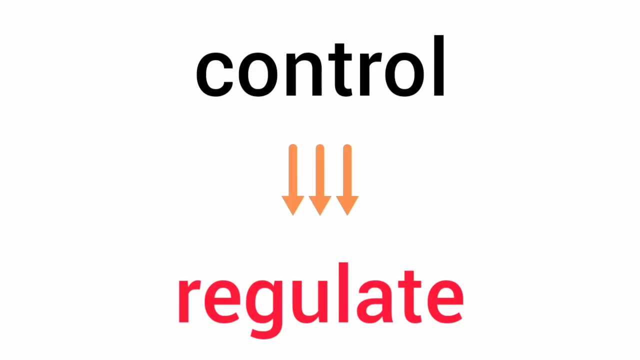 Belly stomach, belly stomach, deceptive, misleading, deceptive, misleading, famous, renowned, famous, renowned. beneficial, Favorable, beneficial, favorable control, regulate, control, regulate fanatic extremist, fanatic extremist, Weird bizarre. 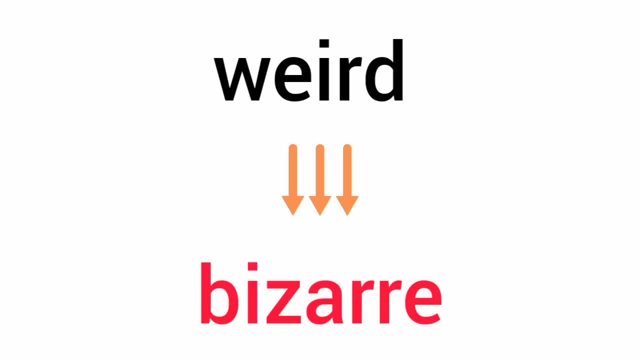 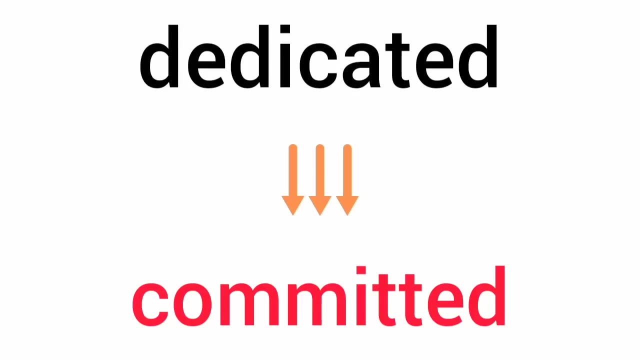 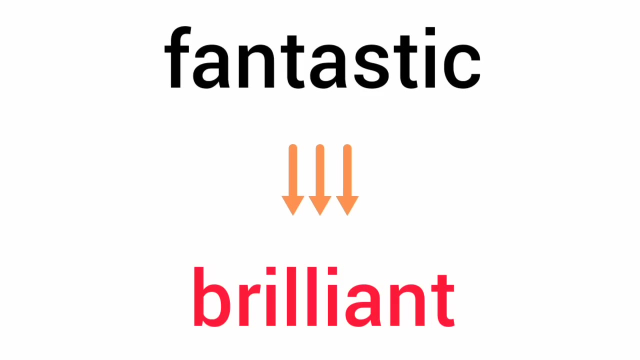 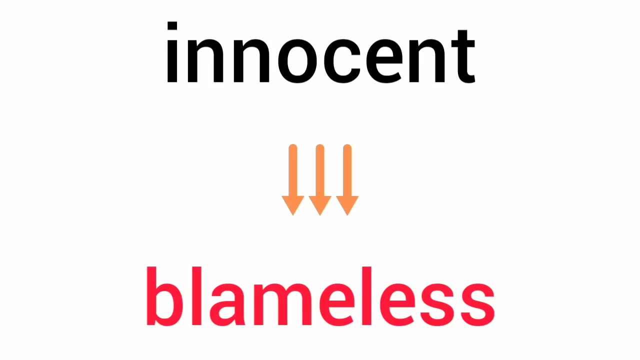 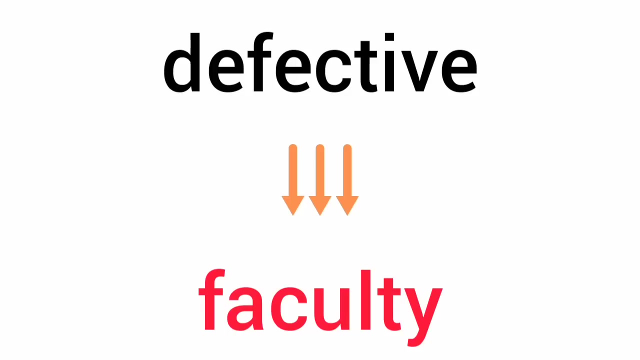 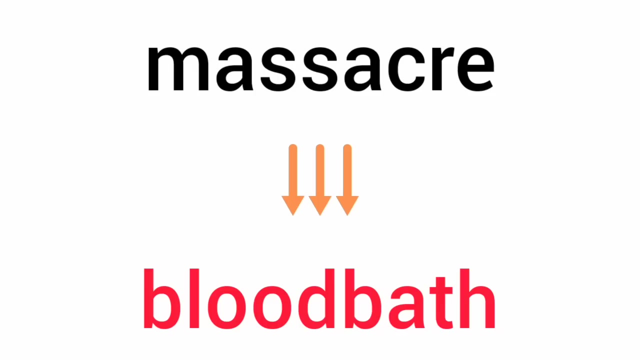 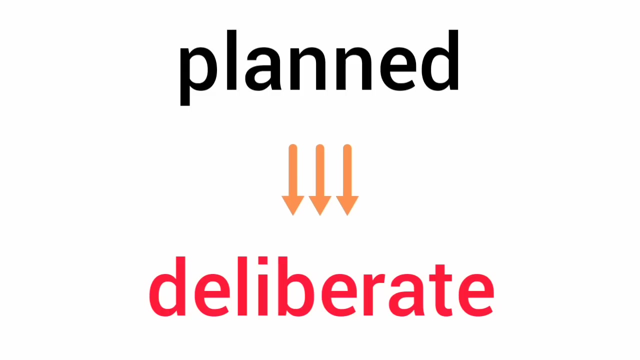 Dedicated, committed, dedicated, committed, Fantastic, brilliant, fantastic, brilliant, Innocent, blameless, innocent, blameless, defective, faulty, defective, faulty drift, float, drift, float, massacre, bloodbath, massacre, bloodbath, planned, deliberate, planned, deliberate, foolish. 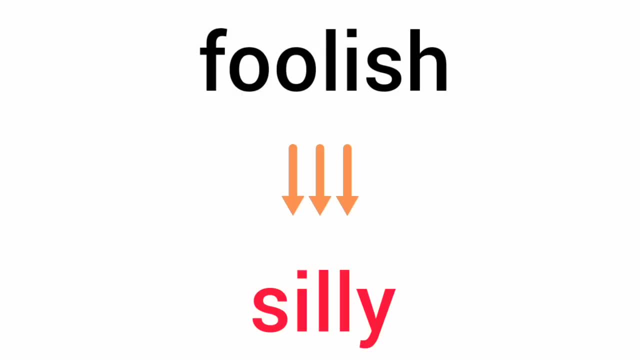 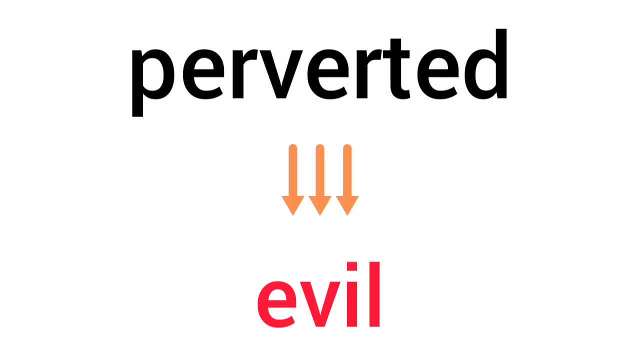 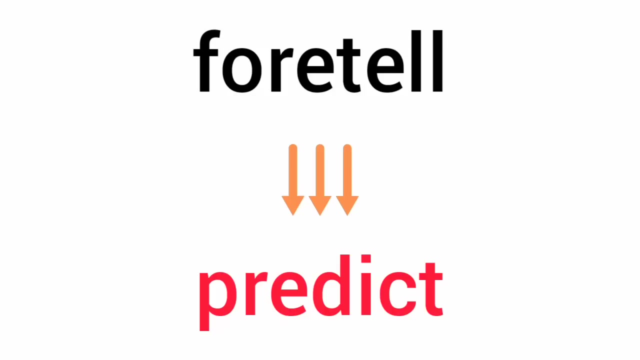 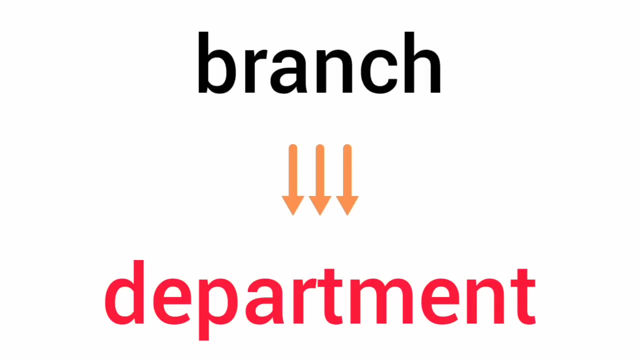 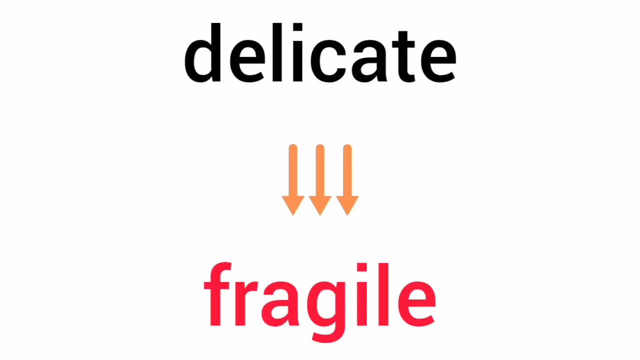 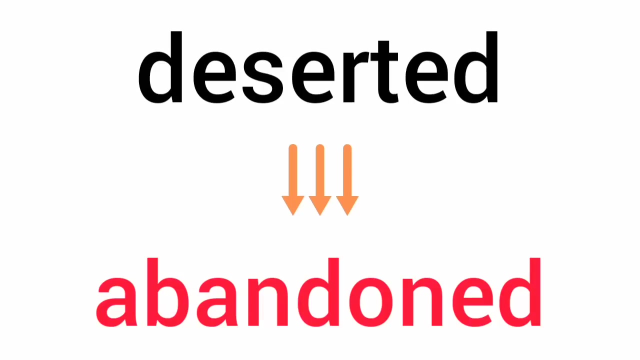 silly, foolish, silly brave, courageous, Brave, courageous. perverted evil, perverted evil. foretell, predict, foretell. predict. branch department, branch department: Delicate, fragile, delicate, fragile, scarce, rare, scarce, rare, deserted, abandoned, deserted. 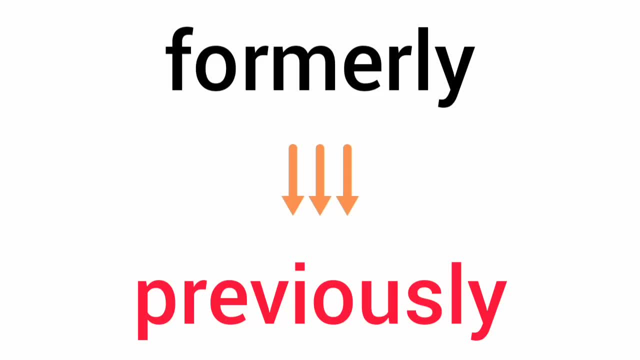 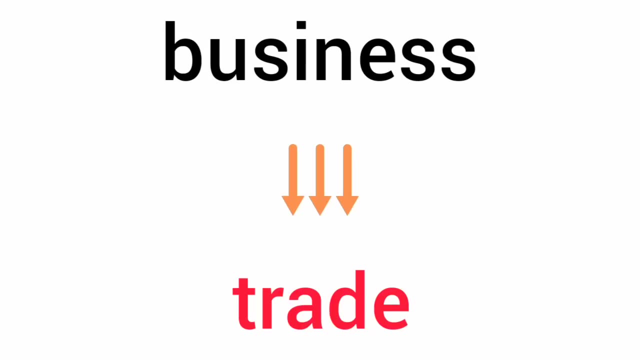 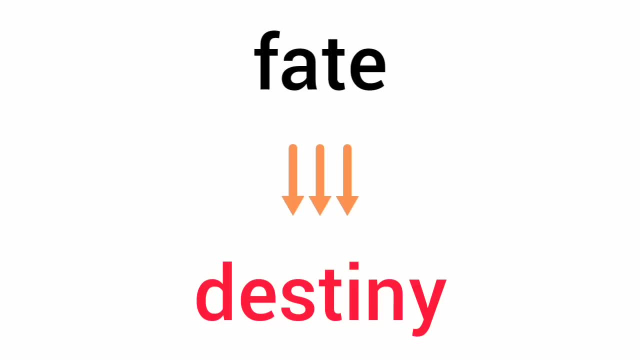 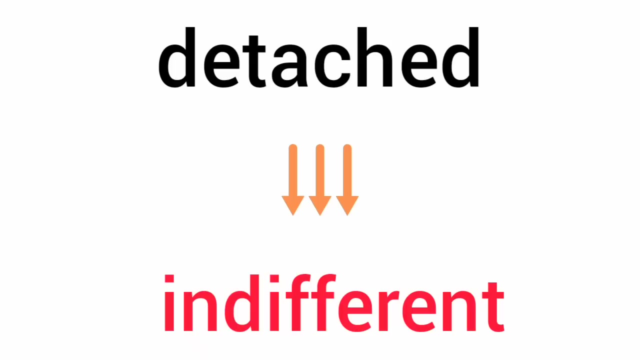 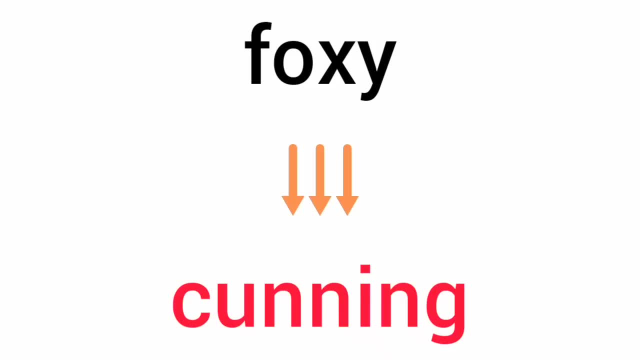 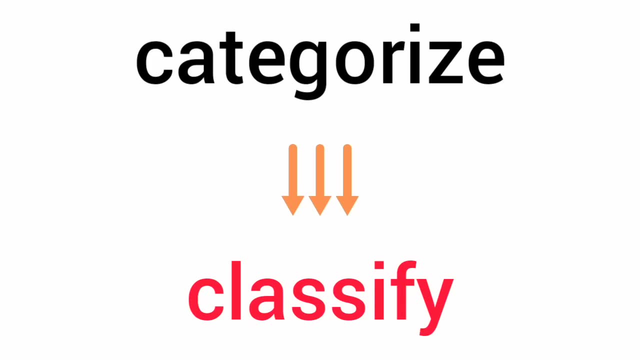 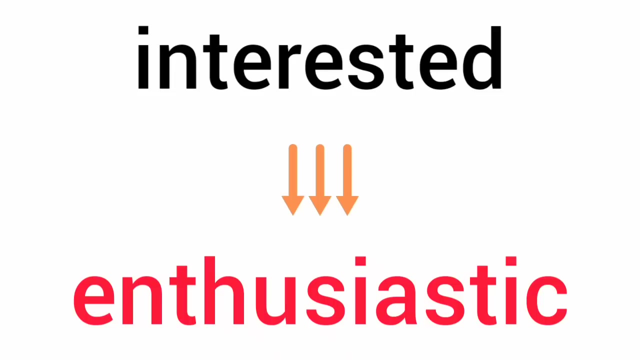 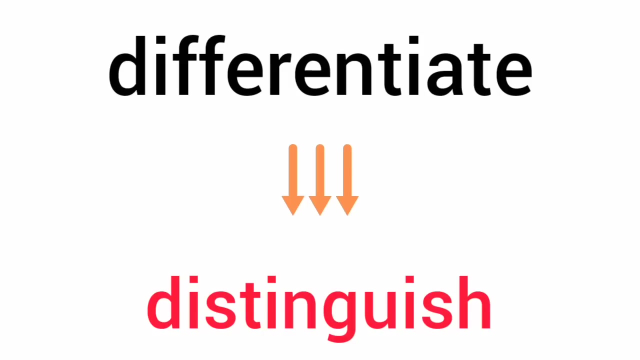 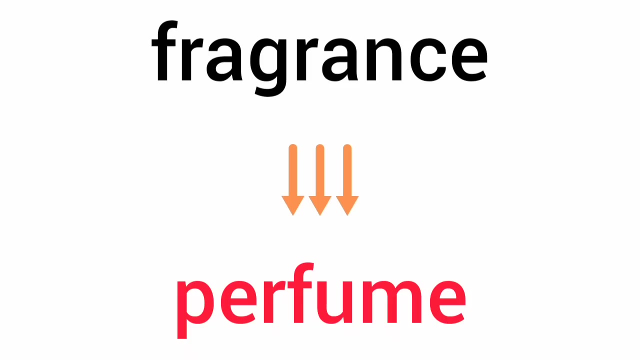 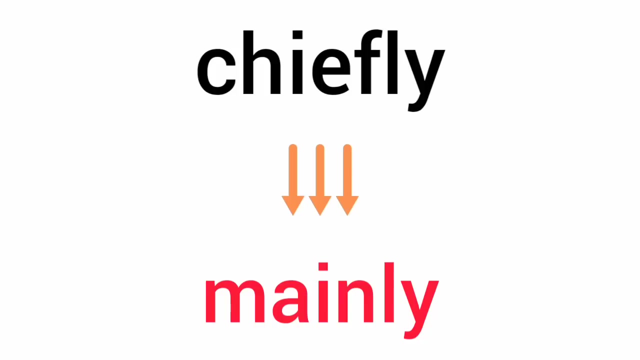 Foxy cunning, foxy cunning. categorize classify. categorize classify Interested: enthusiastic, interested, enthusiastic Differentiate, distinguish differentiate, distinguish Fragrance perfume. fragrance perfume, Chiefly mainly, chiefly, mainly. 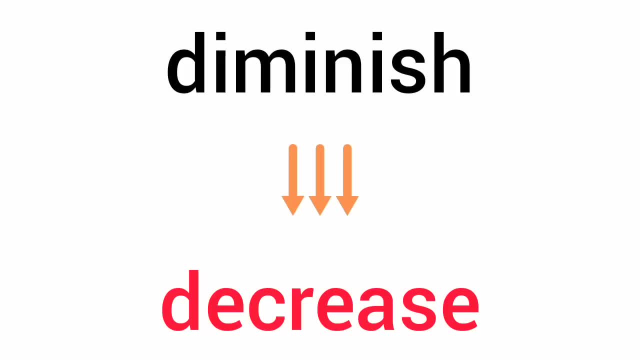 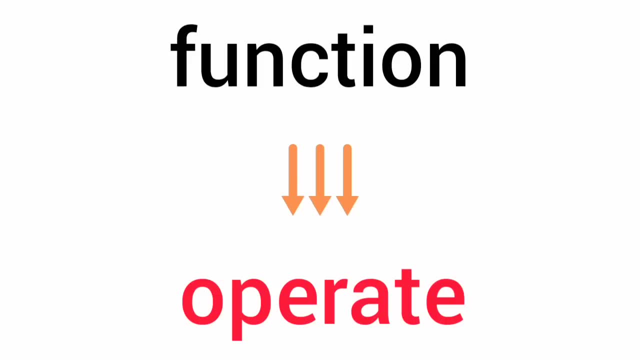 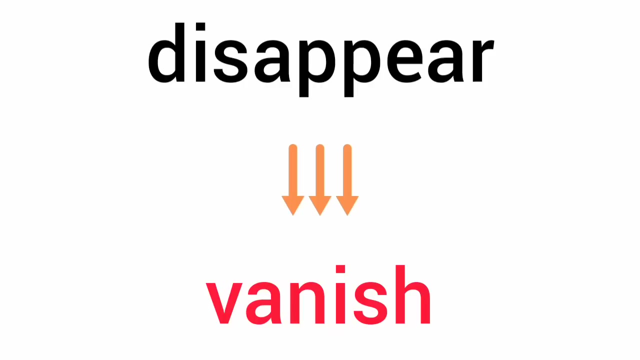 Diminish, Decrease. Diminish, Decrease Function: Operate Function. Operate: Choosy Picky, Choosy Picky. Disappear, Vanish Disappear, Vanish Disappear. 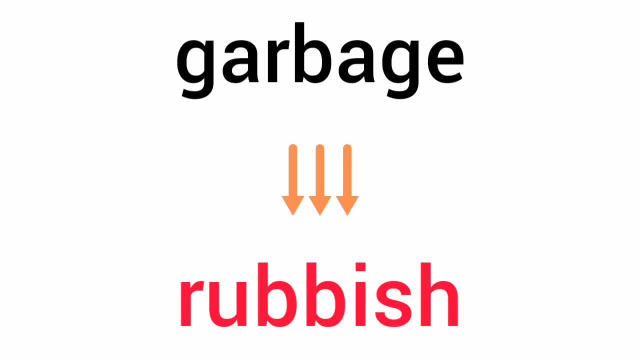 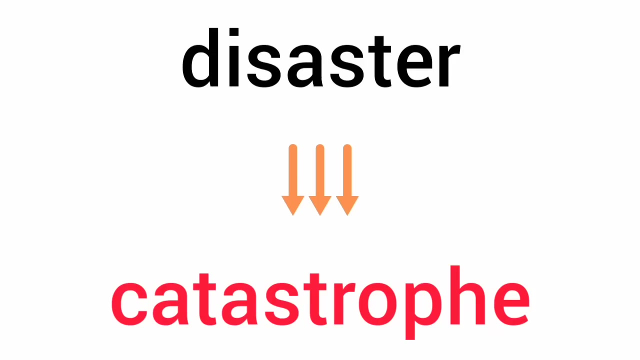 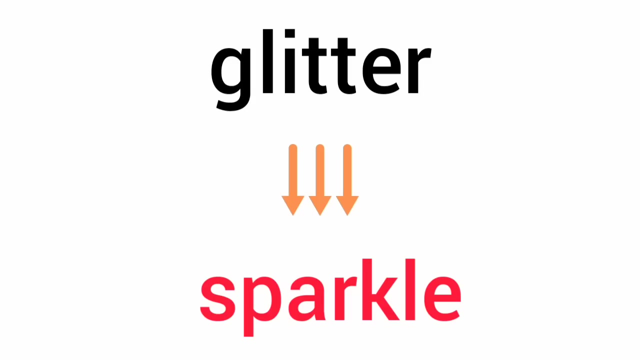 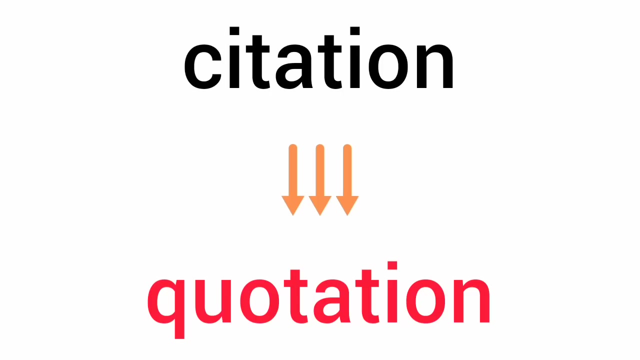 Vanish, Garbage, Garbage, Rubbish, Garbage, Rubbish, Chop, Chop, Chop, Chop. Disaster, Disaster, Catastrophe, Disaster. Glitter, Sparkle, Glitter, Sparkle. Citation Quotation, Citation Quotation. 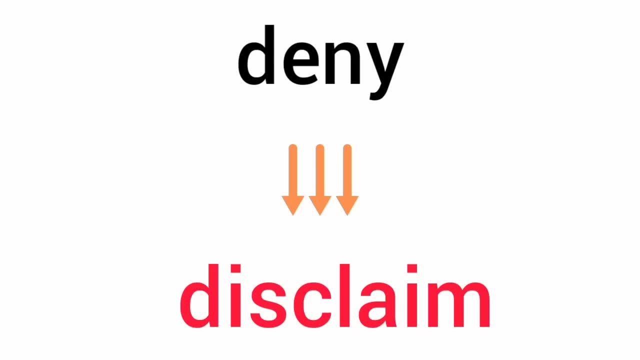 Deny, Disclaim, Deny, Disclaim. Grab Seize, Grab, Seize, Midway, Halfway, Midway, Halfway, Gratis, Free, Gratis, Free. Inflow Incoming Inflow Incoming. 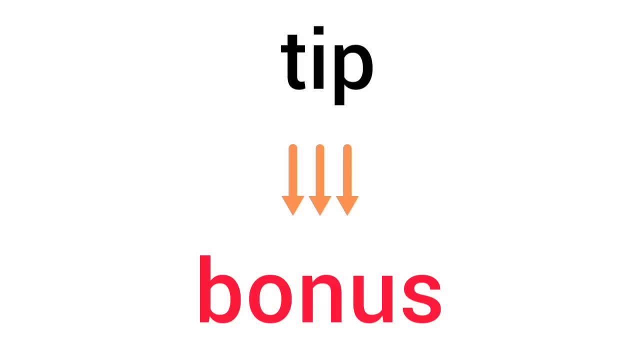 Tip Bonus: Tip Bonus: Casual Informal. Casual Informal, Mild Gentle, Mild Gentle, Intestine, Gut, Intestine Gut, Rare, Infrequent Rare, Infrequent Imitate, Mimic, Imitate. 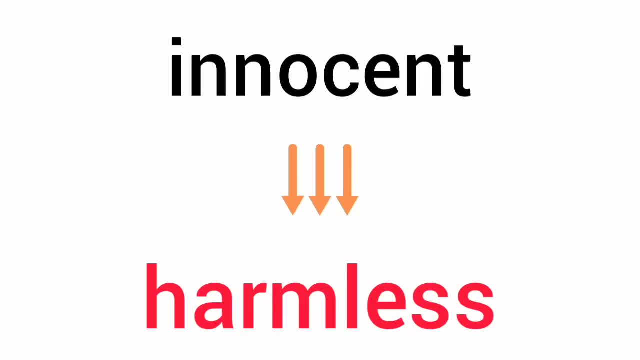 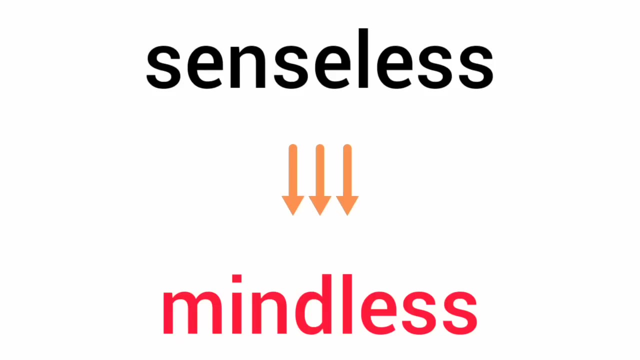 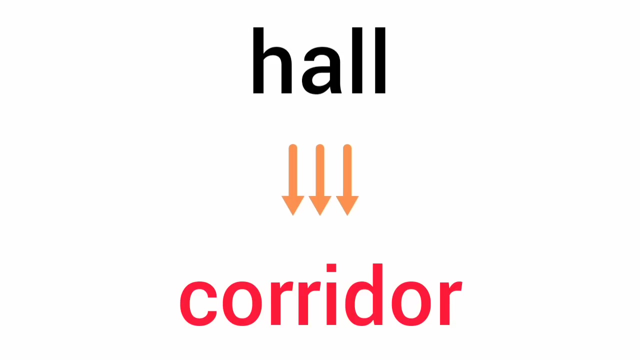 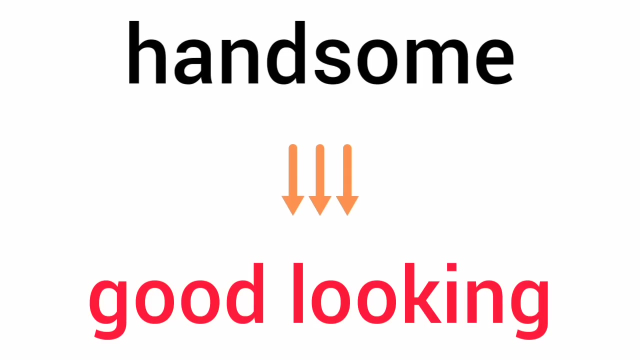 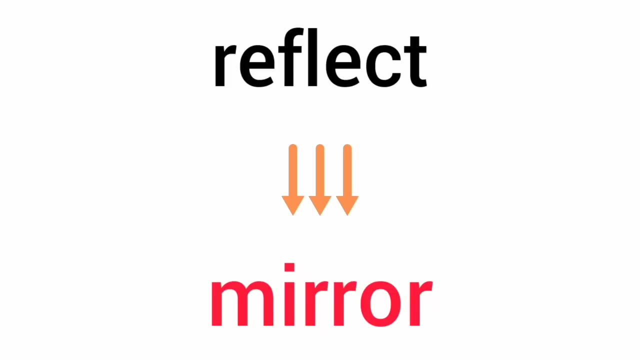 Mimic: Innocent, Harmless, Innocent, Harmless, Senseless, Mindless, Senseless, Mindless, hall corridor, hall, corridor. reduce, minimize, reduce, minimize. handsome, good looking, handsome, good-looking, reflect mirror, reflect mirror. happy, joyful, happy, joyful instinct, intuition, instinct. 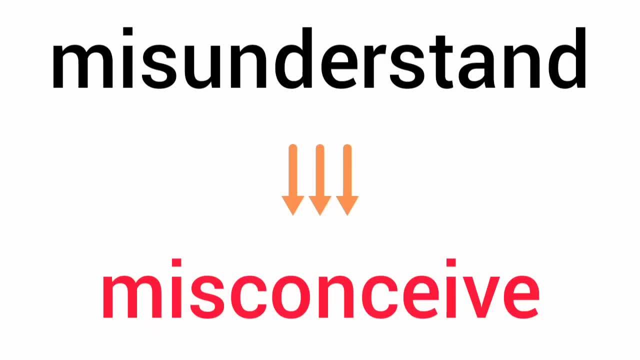 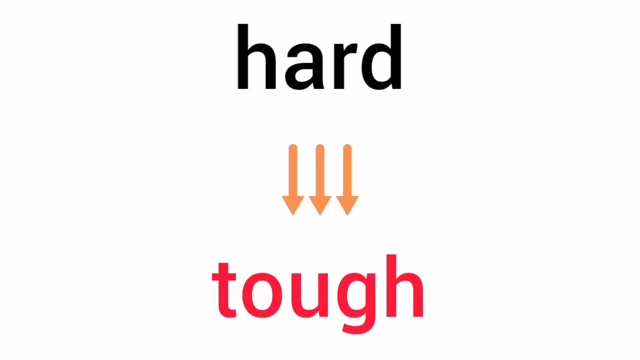 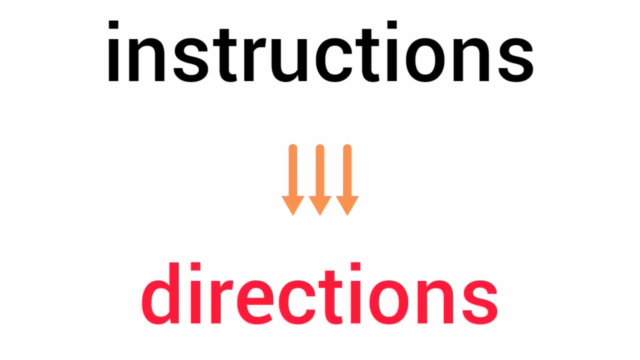 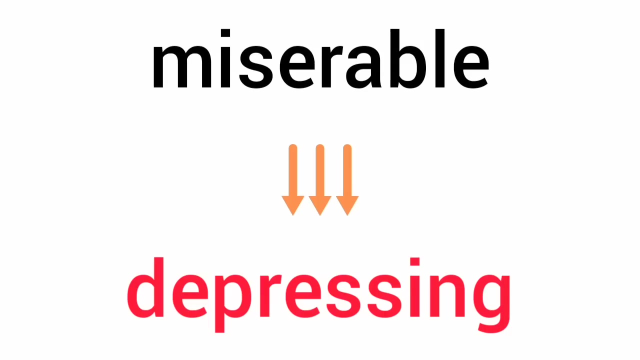 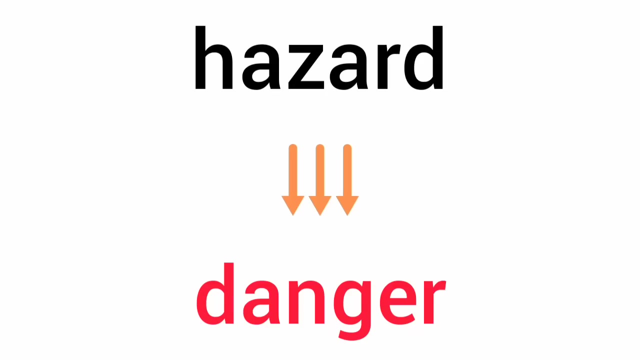 intuition: Misunderstand, misconceive, Misunderstand, misconceive. Hard, tough, Hard, tough. Instructions, directions, Instructions, directions. Miserable, depressing, Miserable, depressing, Hazard, danger, Hazard danger. 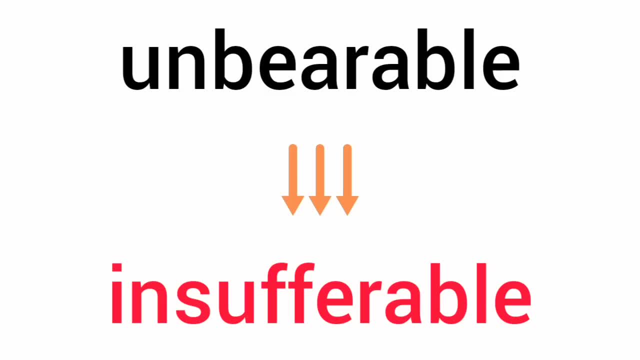 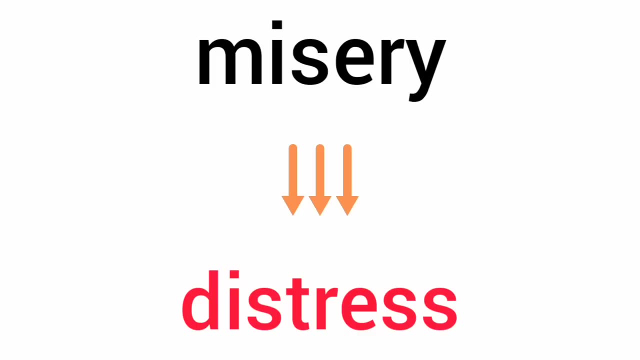 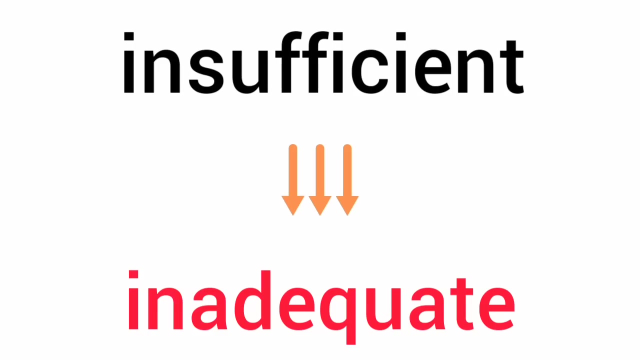 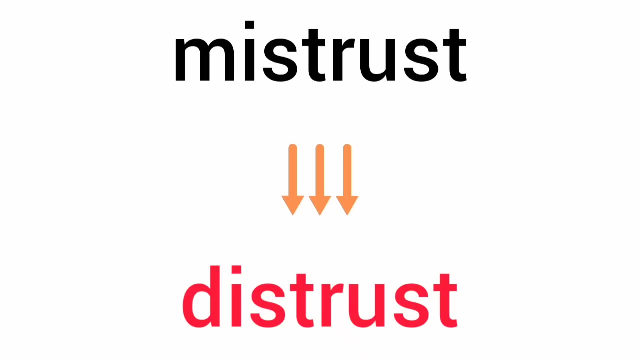 Unbearable, insufferable, Unbearable, insufferable, Misery, distress, Misery, distress, Rumour, rumor, Insufficient, inadequate, Insufficient, inadequate. Mistrust, distrust, Mistrust, distrust. 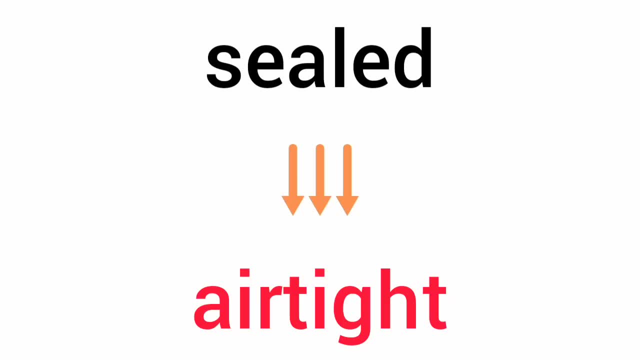 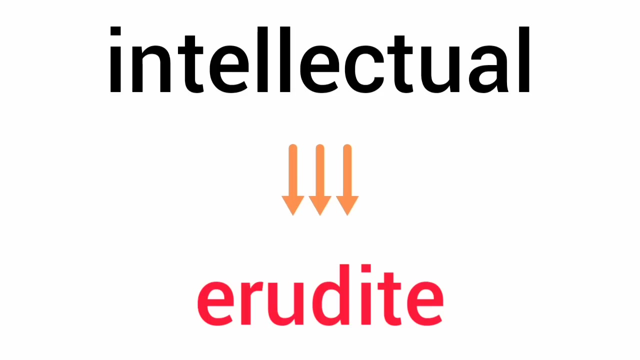 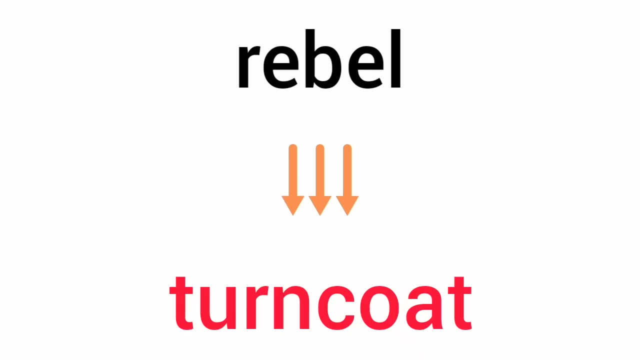 Sealed airtight, Sealed airtight. More increasing, More increasing. Intellectual erudite. Intellectual erudite: Rebel torn coat, Rebel torn coat, Movie, film, Movie, film. Tell hint, Tell hint. Intensify, heighten, Intensify, heighten. 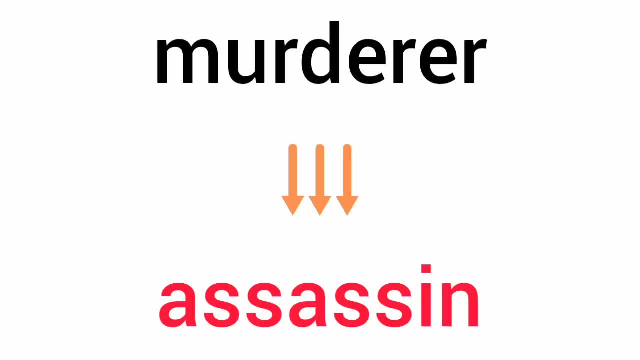 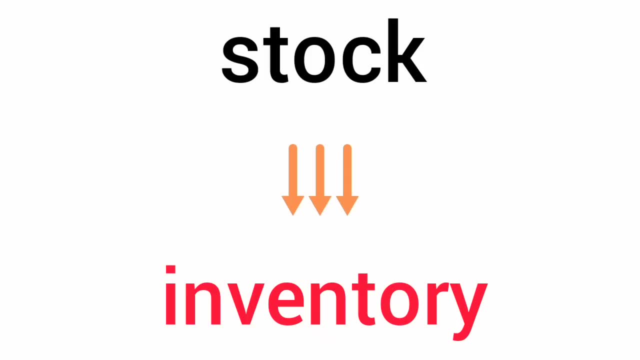 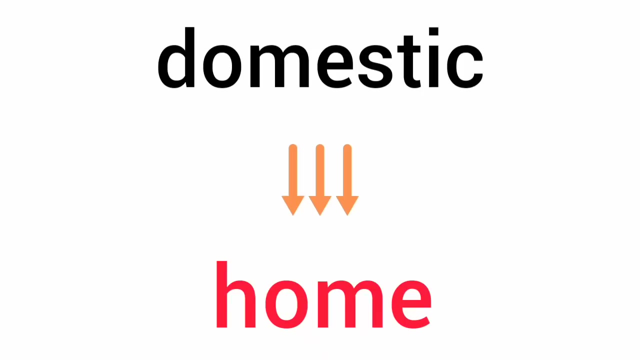 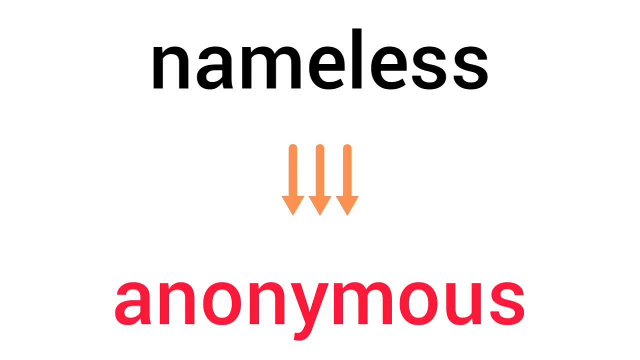 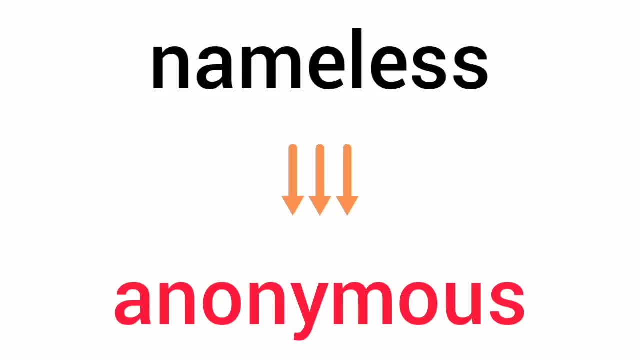 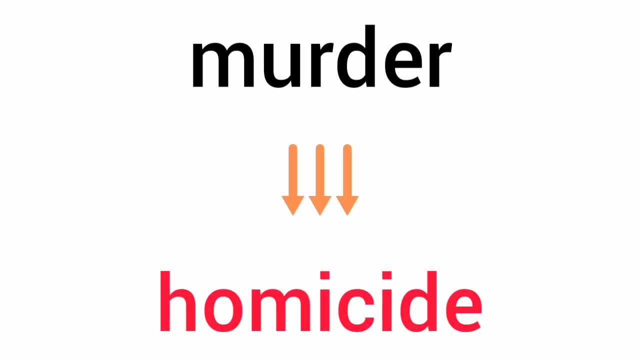 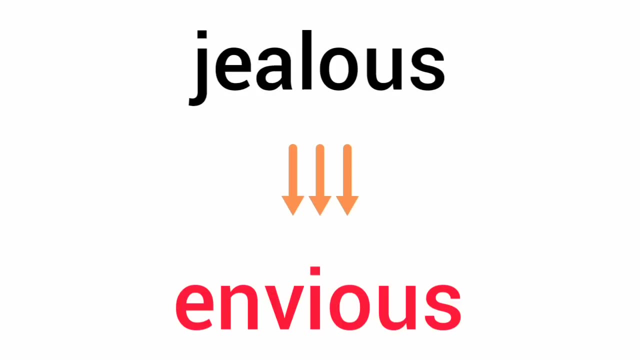 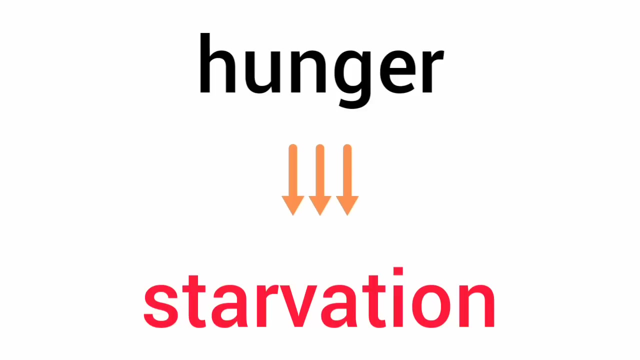 Anonymous, Nameless Anonymous, Murder, Homicide, Murder, Homicide, Jealous Envious, Jealous Envious. Napkin, Serviette, Napkin, Serviette, Hunger, Starvation, Hunger, Starvation. 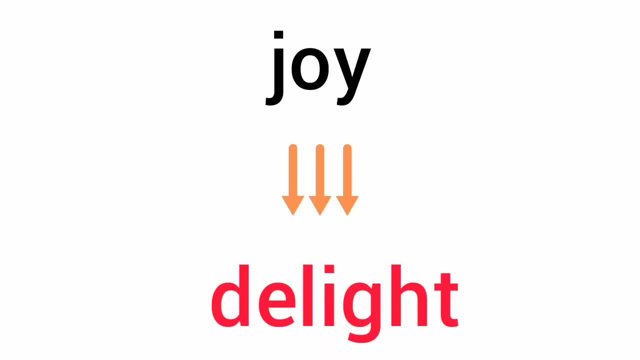 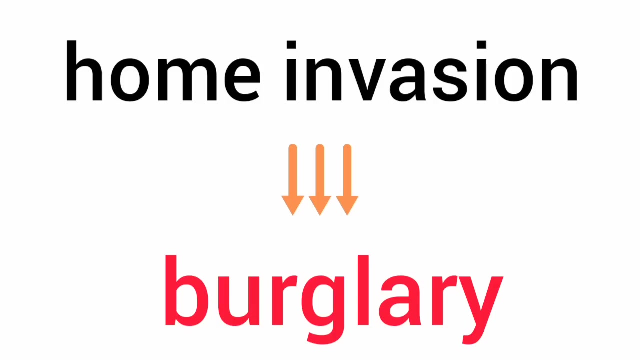 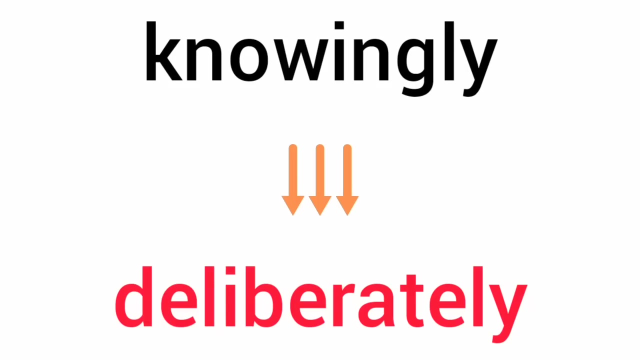 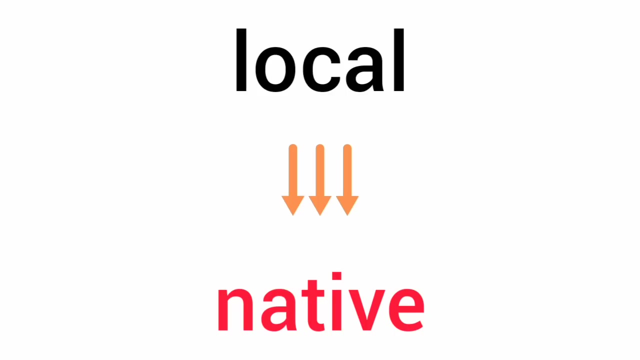 Joy Delight, Joy Delight. Story Narrative. Story Narrative: Home invasion. Home invasion, burglary. Home invasion, burglary. Knowingly, Deliberately, Knowingly Deliberately, Local Native Had. 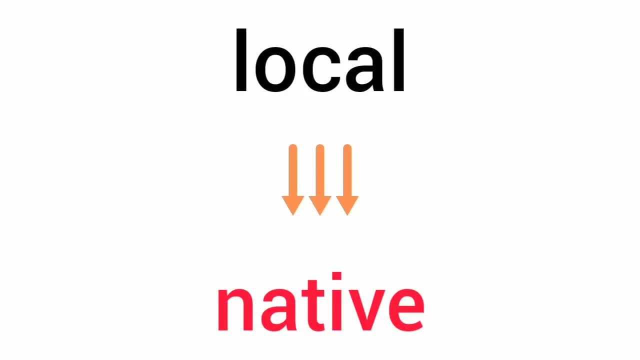 Local Exèrcit, Legendary Iconic Prom Normal Needs ComALKIMOLOGISTA OCH investigative media. aKing smb read otterca 했byadrudeet Rush, hurry, Rush, hurry. Missing, lacking. 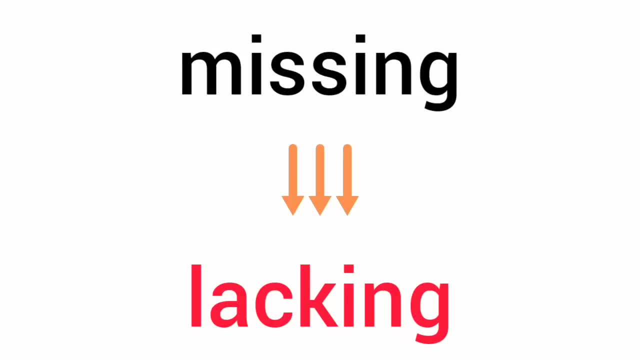 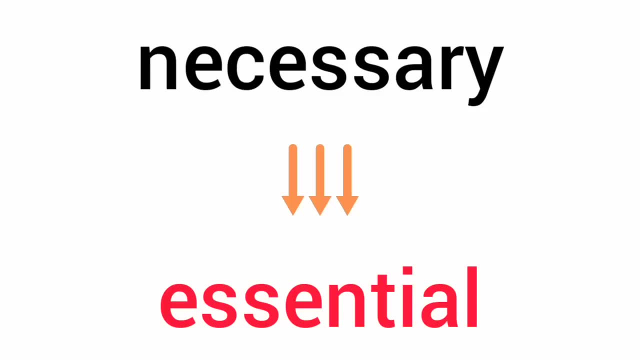 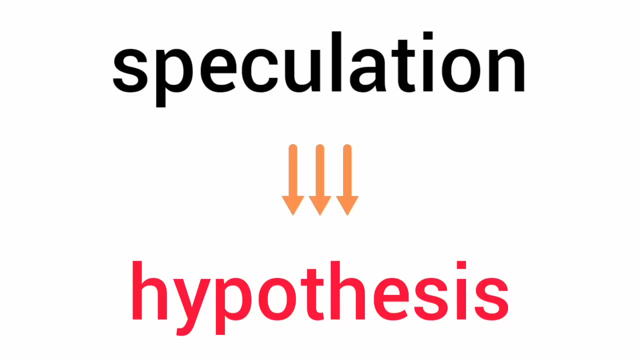 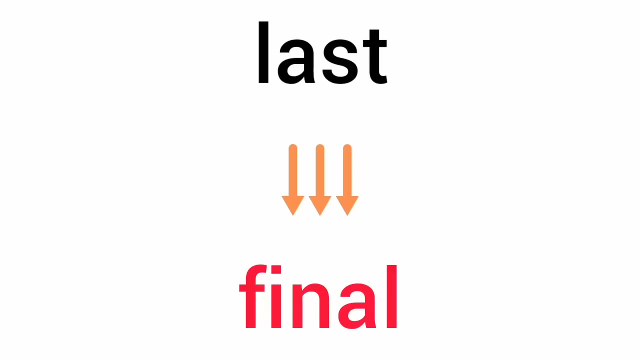 Missing, lacking, Necessary, essential, Necessary, essential. Speculation hypothesis: Speculation hypothesis: Last final, Last final. Dusk nightfall, Dusk nightfall, Weather Weather, If, whether, If Leader chief Leader, chief Appoint nominate, Appoint nominate. 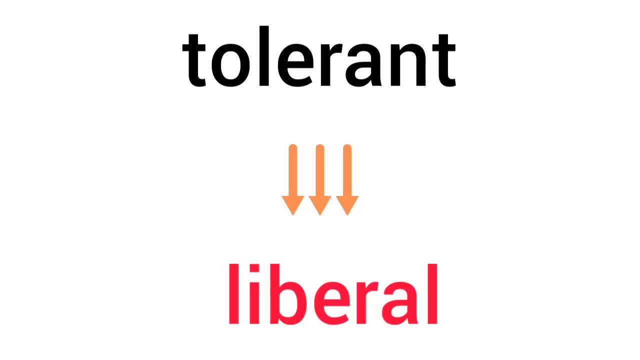 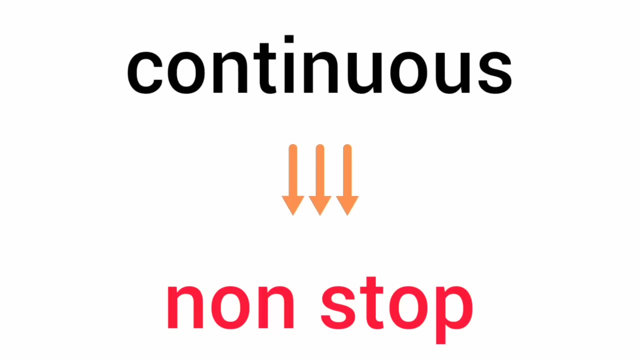 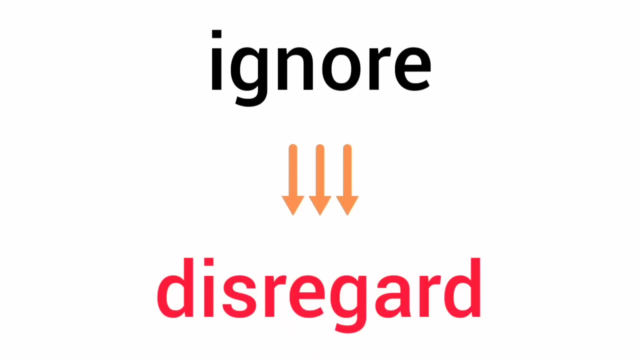 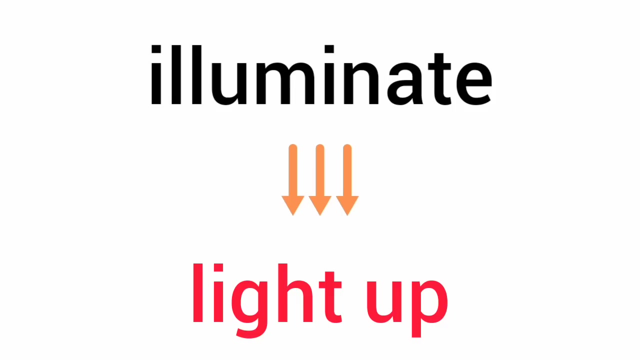 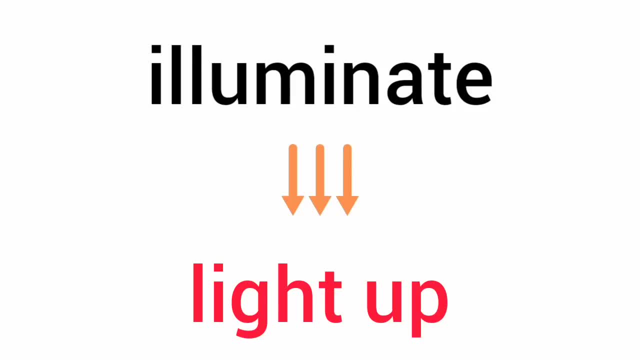 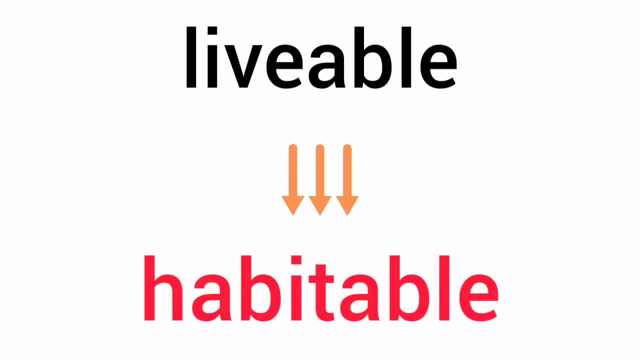 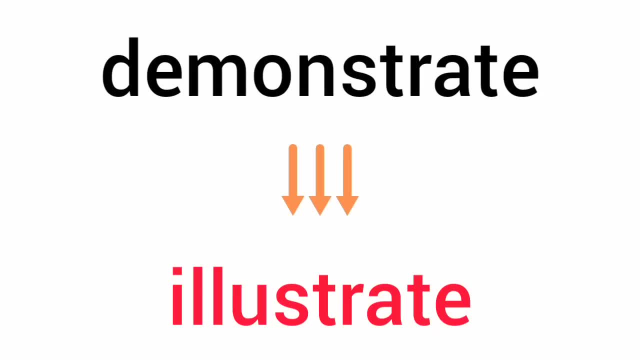 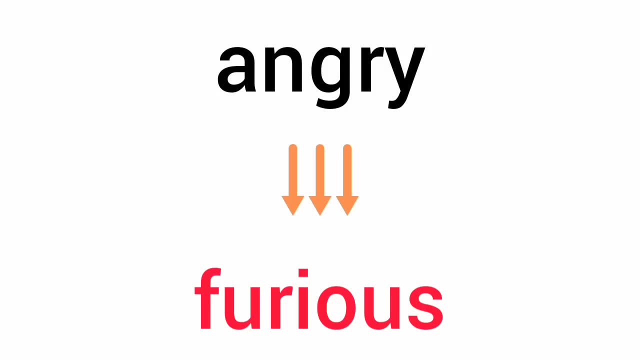 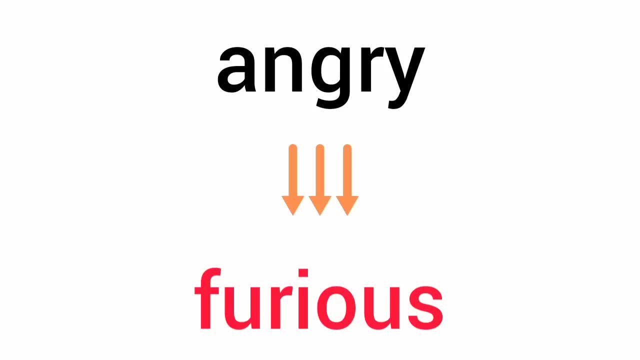 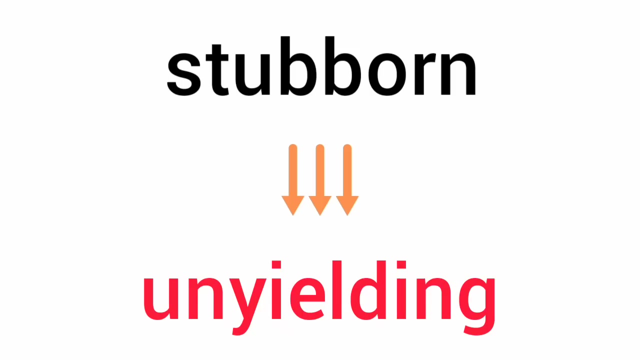 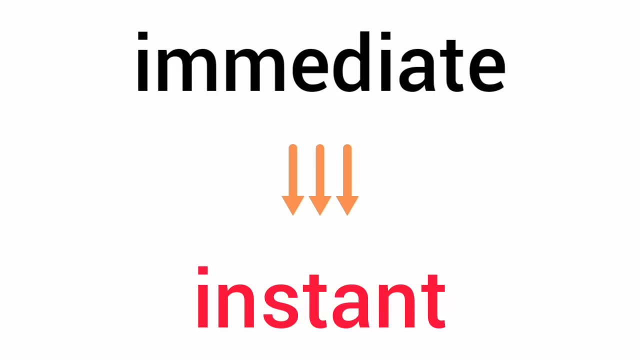 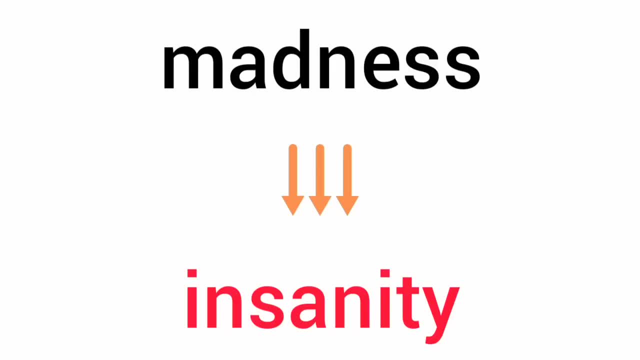 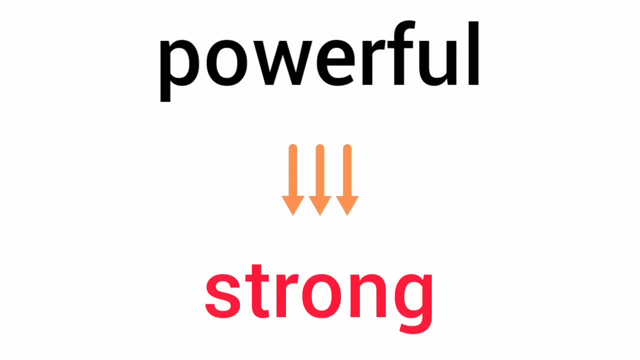 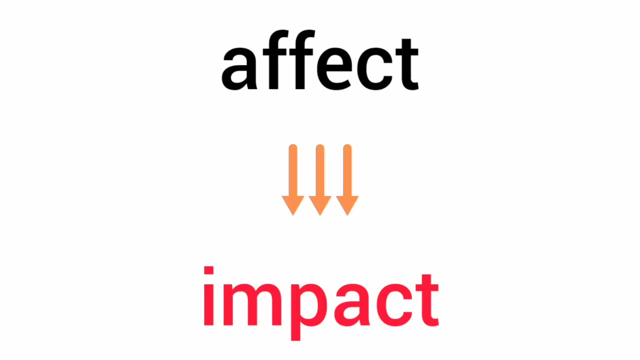 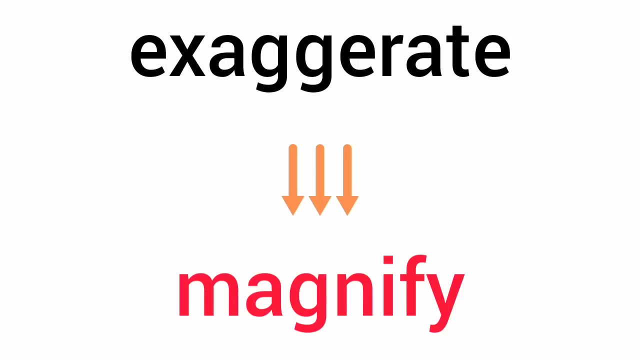 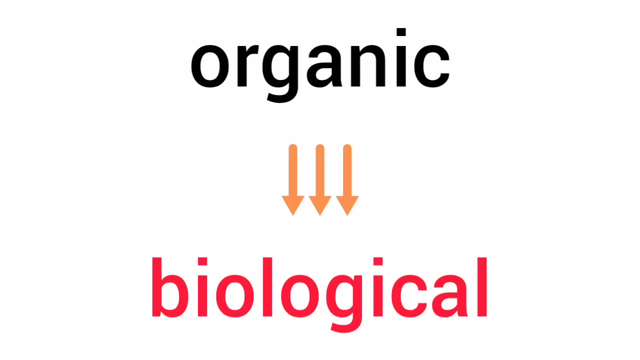 Insanity, Madness, Insanity, Powerful, Strong, Powerful, Strong, Affect, Impact, Affect, Affect, Impact. Exaggerate, Magnify, Exaggerate, Magnify. Organic Biological. Organic Biological. 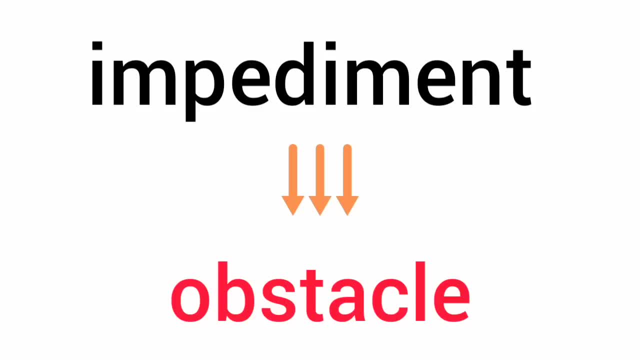 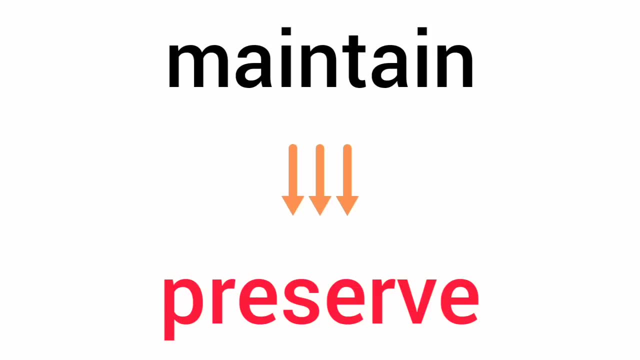 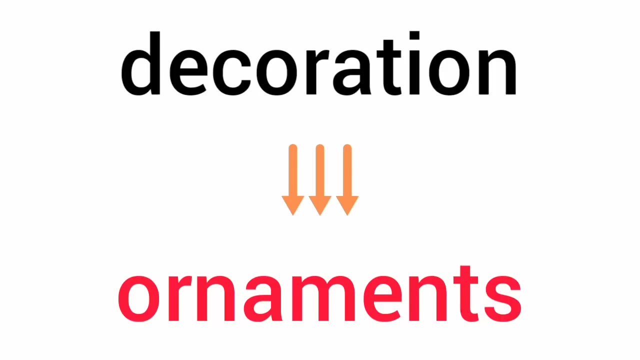 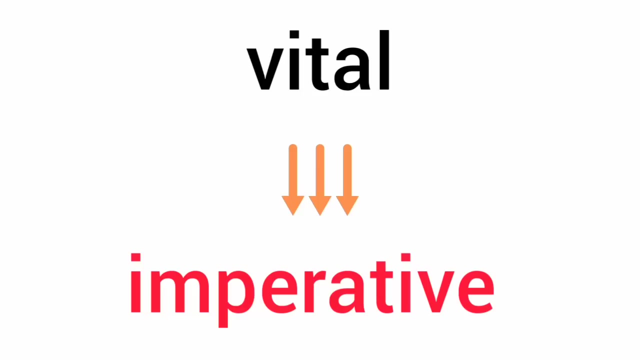 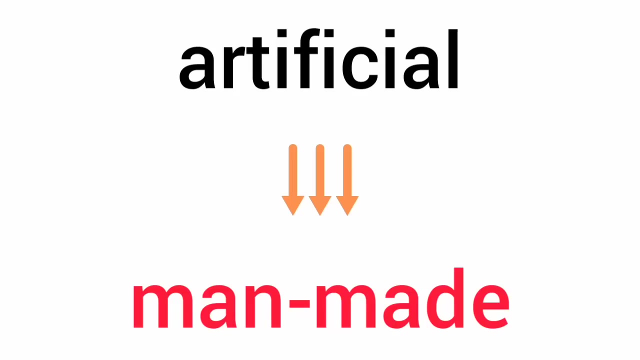 Impediment, Obstacle, Impediment, China, impediment, obstacle, maintain, preserve, maintain, preserve. decoration, ornament, ornament, decoration, ornament, vital imperative, vital imperative, artificial man-made, artificial man-made outside external. 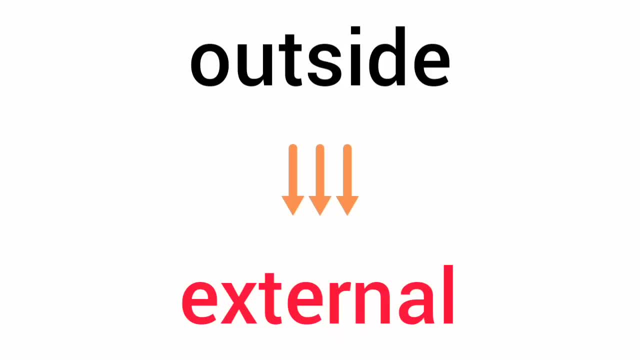 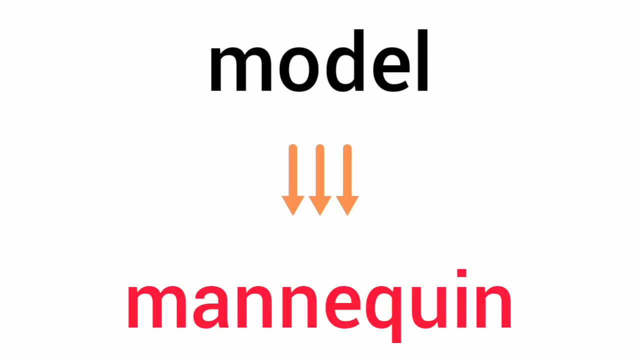 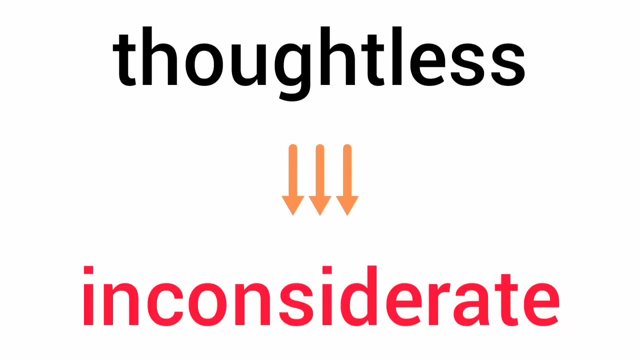 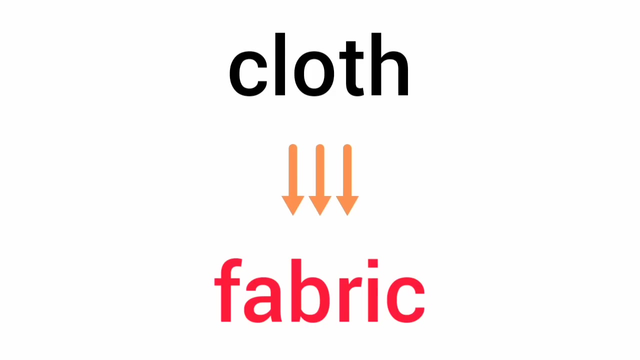 Outside, external: rude, impolite, rude, impolite model, mannequin model, mannequin, neglect, overlook neglect. Thoughtless, inconsiderate, thoughtless, inconsiderate. cloth fabric, cloth fabric. 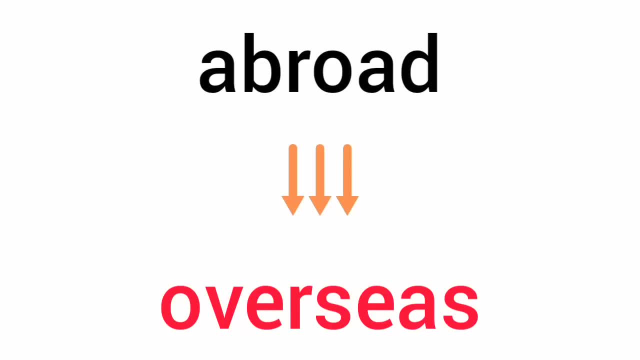 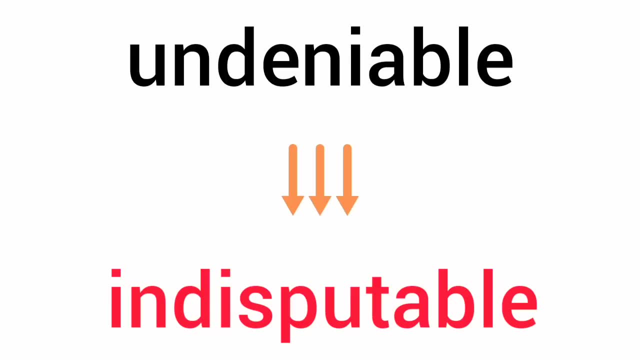 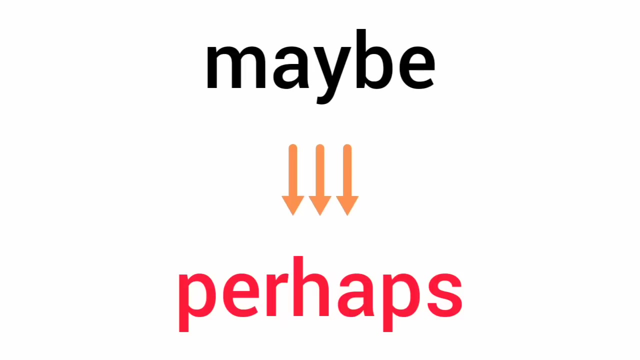 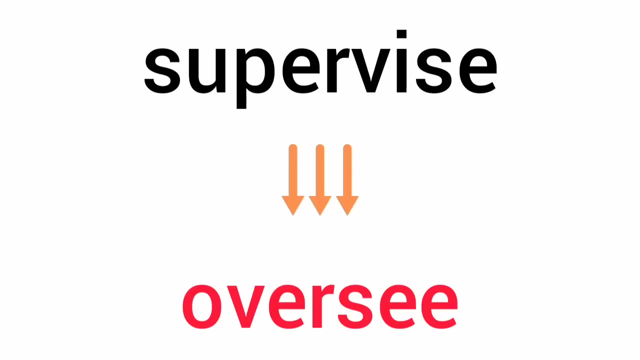 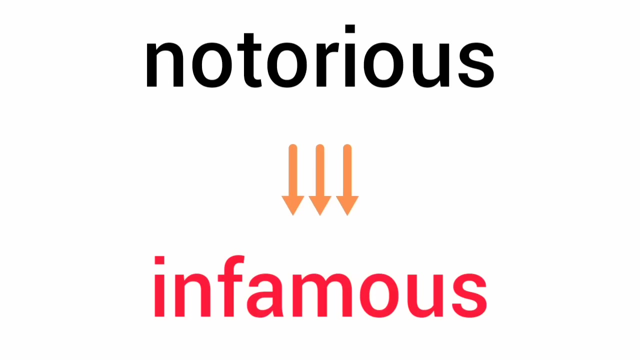 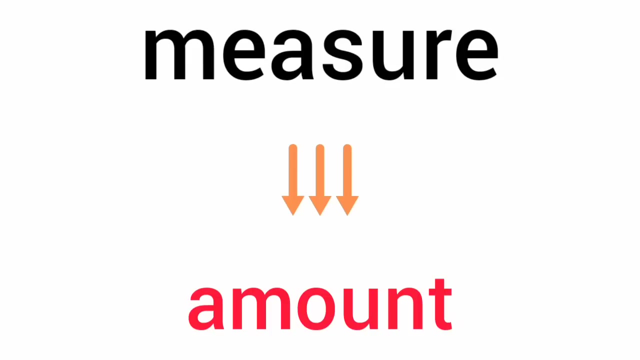 Abroad, overseas, abroad, overseas, Develop Throw Undeniable, indisputable, Undeniable, indisputable, Maybe, perhaps, Maybe, perhaps, Supervise, oversee, Supervise, oversee. Notorious, infamous, Notorious, infamous. Measure amount, Measure amount. 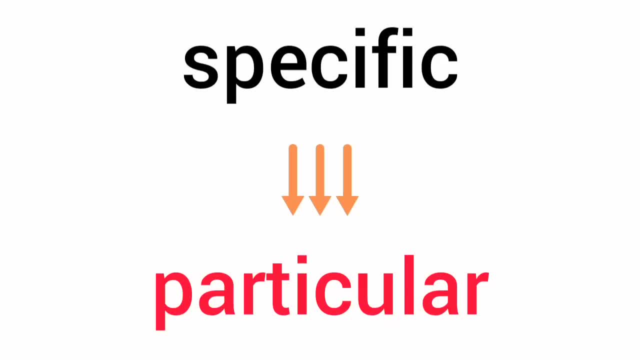 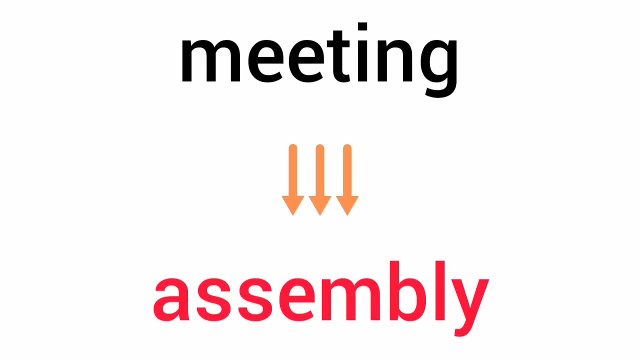 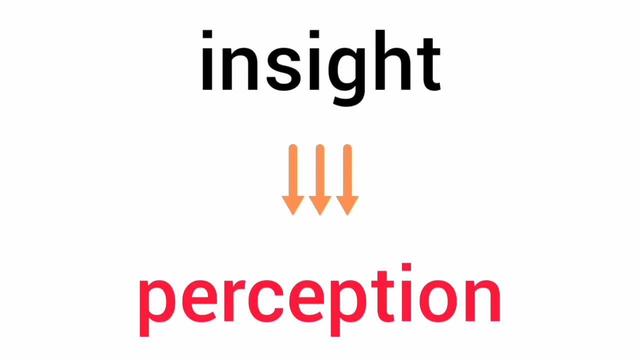 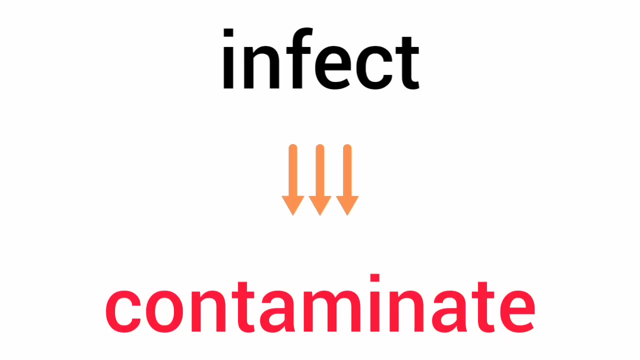 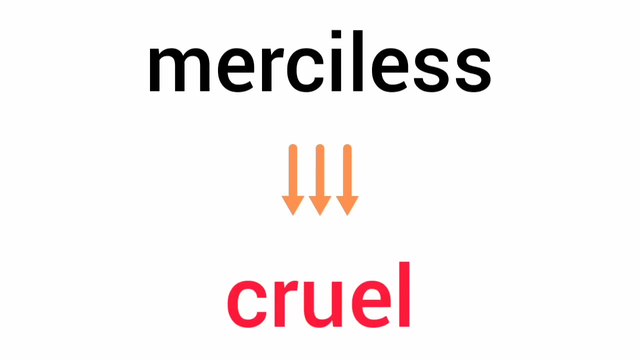 Specific, particular Measure amount. Specific particular Childish puerile- Childish puerile Meeting assembly, Meeting assembly: Insight perception: Insight perception. Insight perception. Infect contaminate, Infect, contaminate, Merciless, cruel, Merciless, cruel. 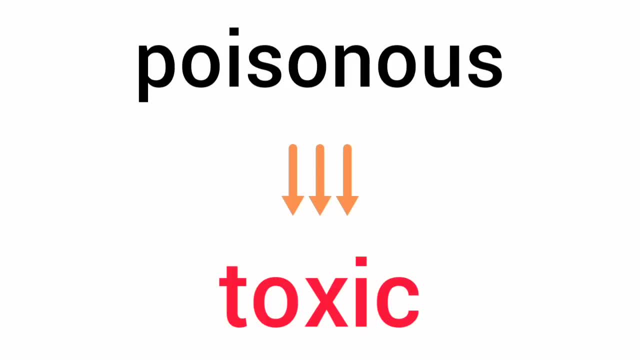 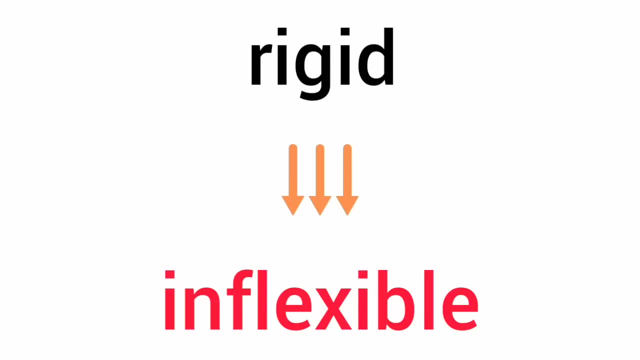 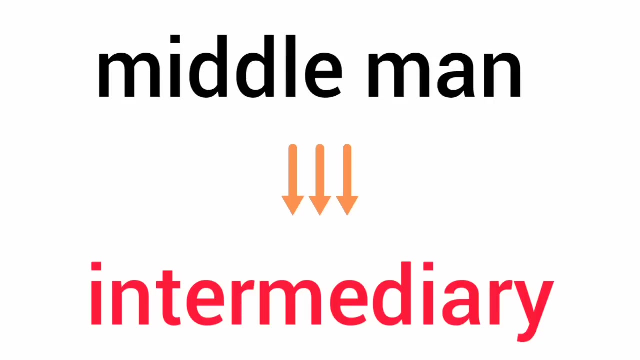 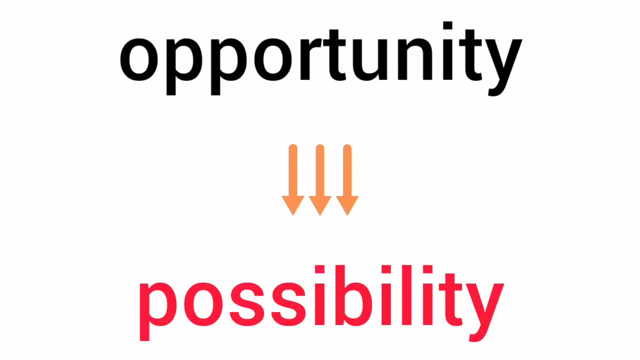 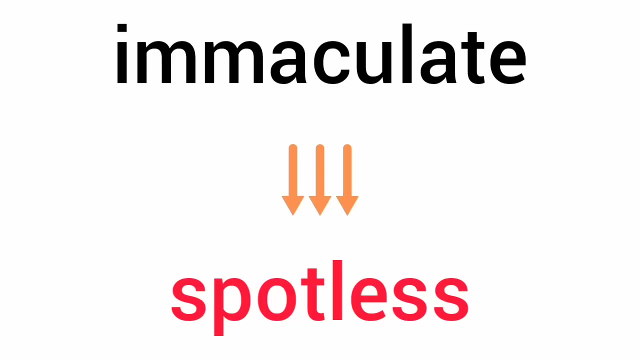 Merciless, cruel, Poisonous, toxic, Poisonous toxic, Poisonous toxic, Rigid, inflexible, Rigid, inflexible. Middle man intermediary, Middle man intermediary. Opportunity, possibility, Opportunity, possibility, Immaculate spotless, Immaculate spotless. 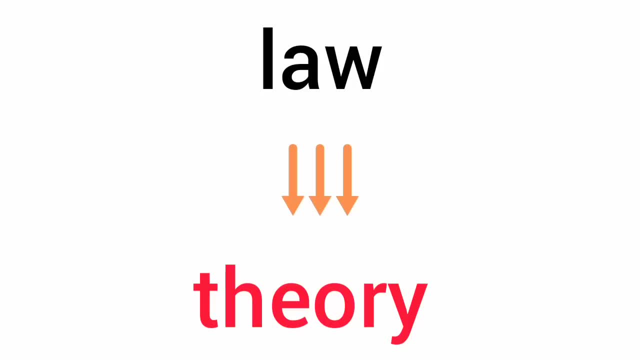 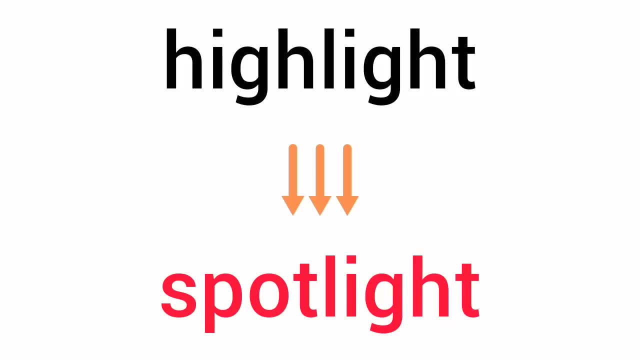 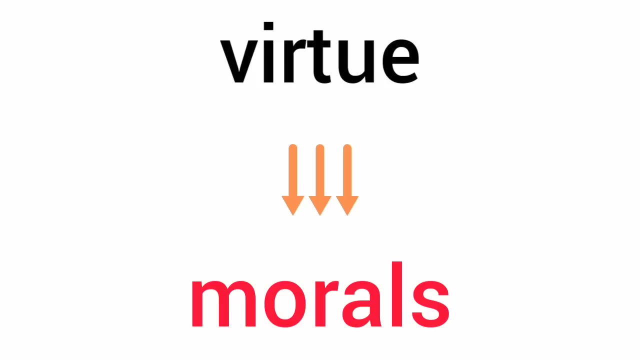 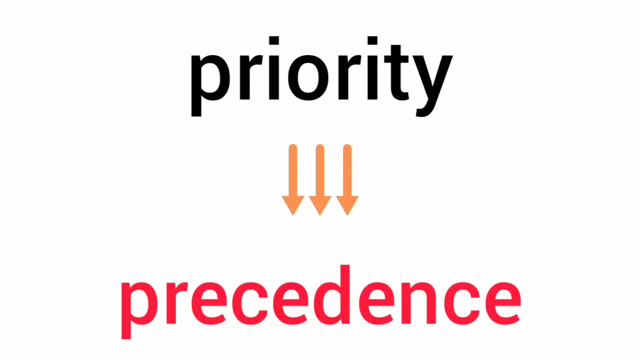 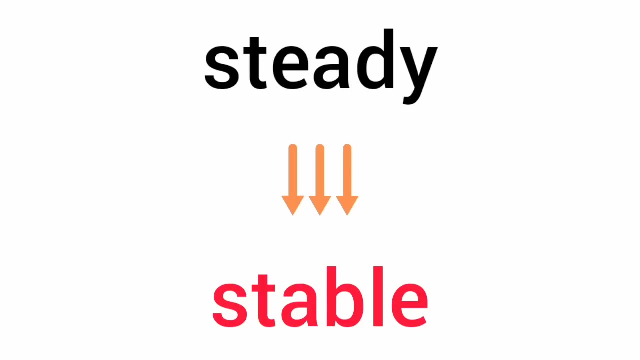 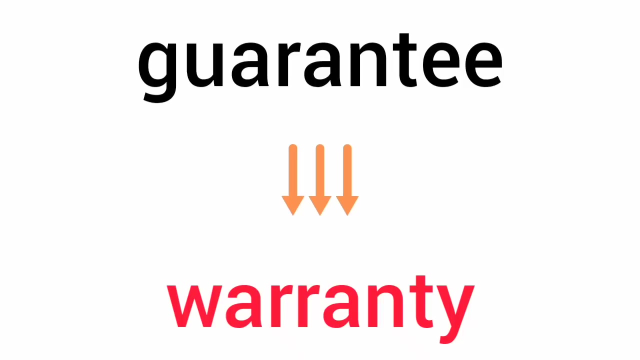 Law theory: Law theory: Highlight, spotlight, Highlight, spotlight. Virtue Morals, virtue morals: priority, precedence, priority precedence. steady, stable, steady stable, silly, stupid, silly, stupid. guarantee, warranty, guarantee, warranty. imagine, visualize: 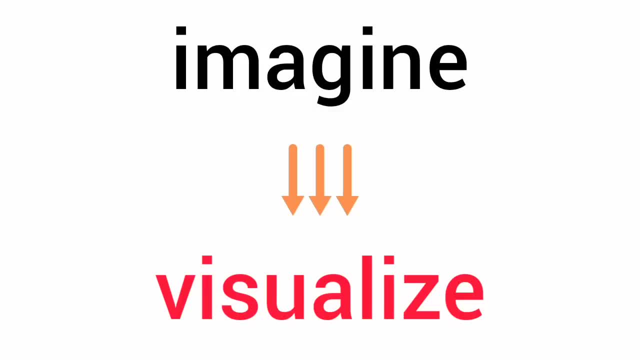 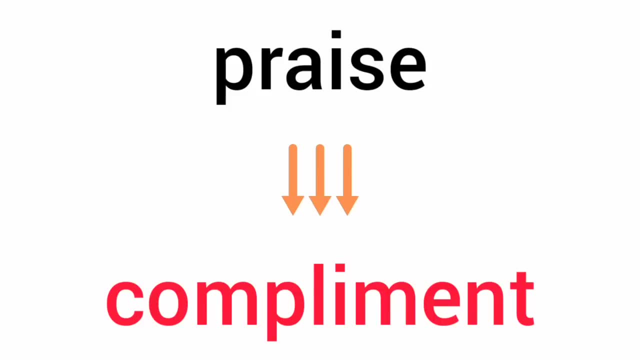 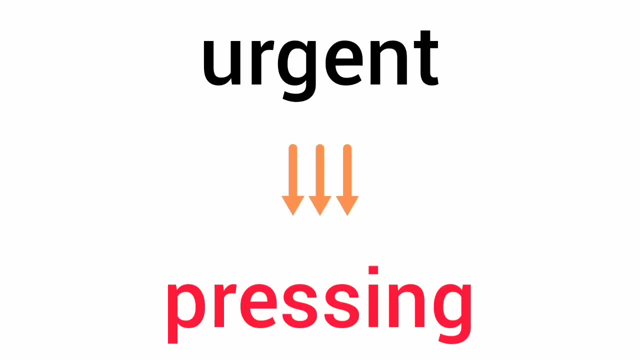 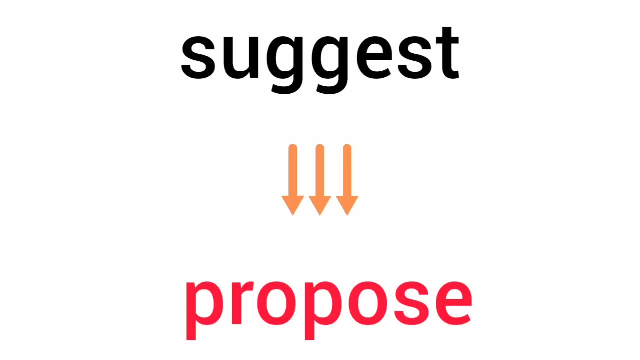 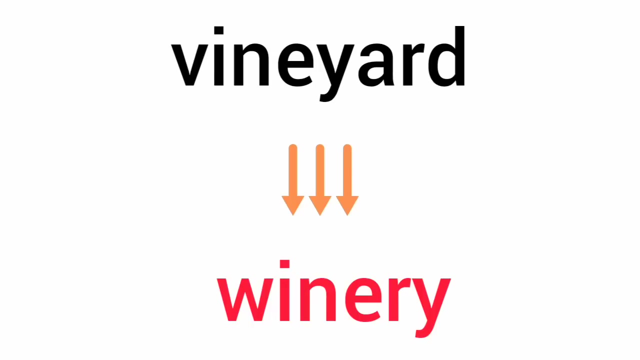 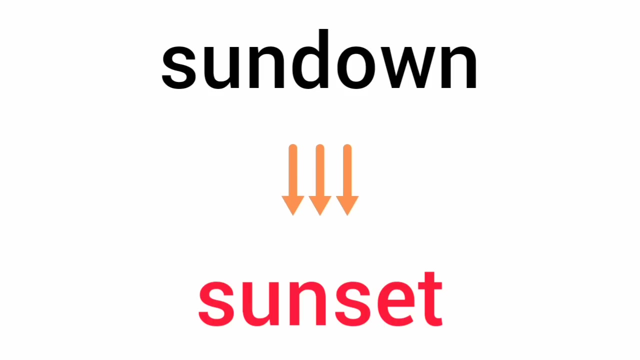 imagine: Praise, compliment, praise, compliment, urgent pressing, urgent pressing, suggest, propose, suggest propose. Vineyard winery. vineyard winery, previous former. previous former sundown, sunset. 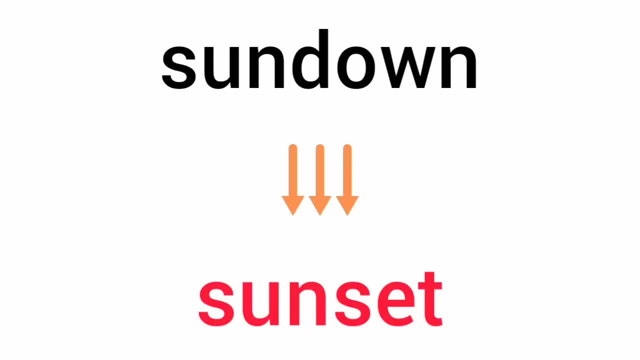 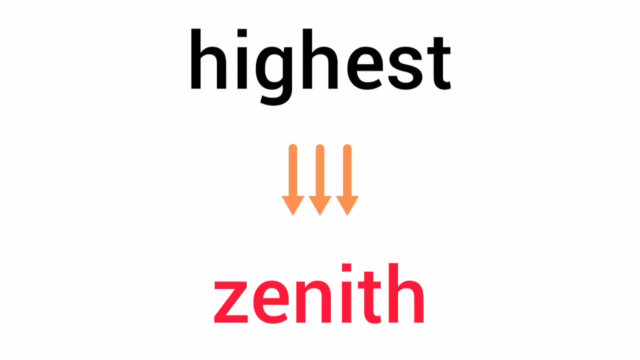 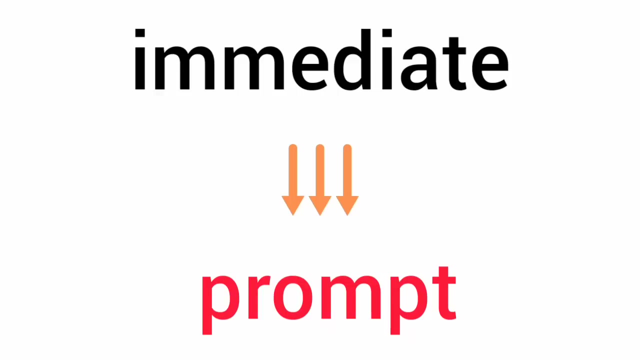 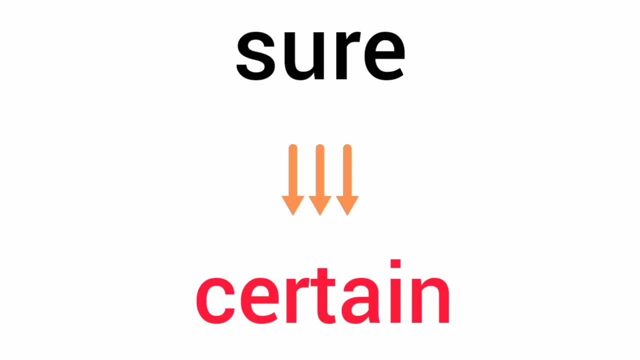 sunset, sundown, sunset, dawn, Sunrise, dawn, sunrise, withstand, resist, withstand, resist. highest zenith, highest zenith immediate, prompt, Sure, certain, sure, certain, Calm approach, calm approach, rich affluent, rich affluent. 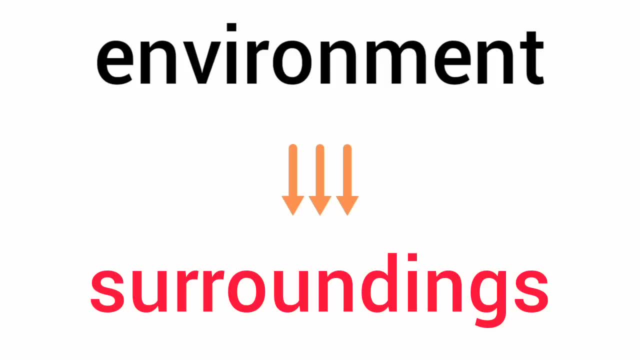 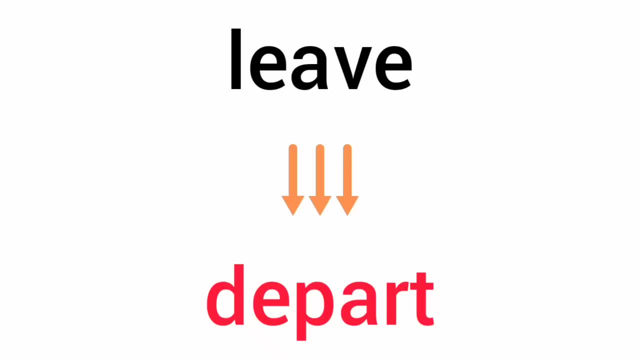 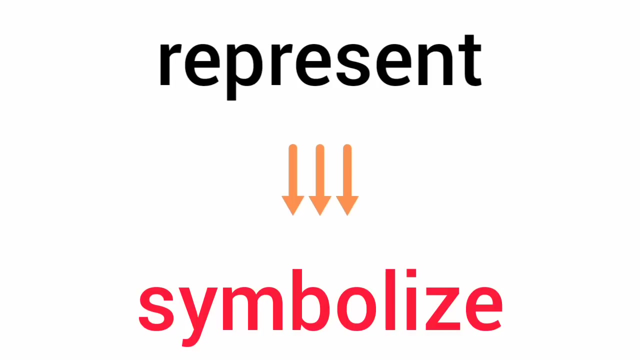 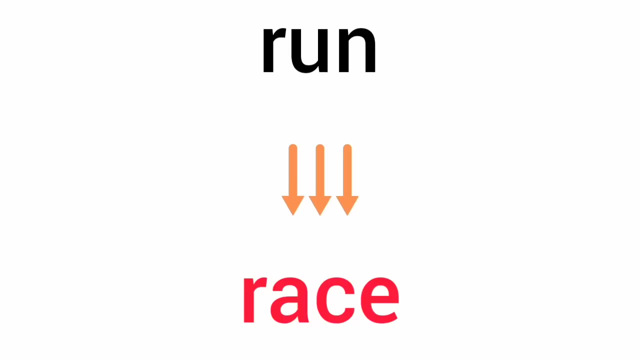 environment, surroundings, environment surroundings. leave depart, leave depart, provide supply, provide supply. represent symbolize, represent symbolize. run, race, run, race, tremble, shiver, tremble. 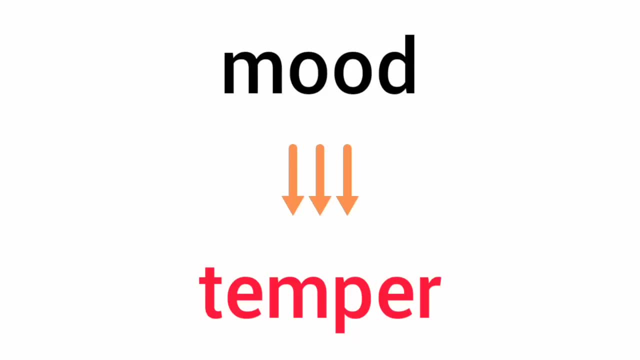 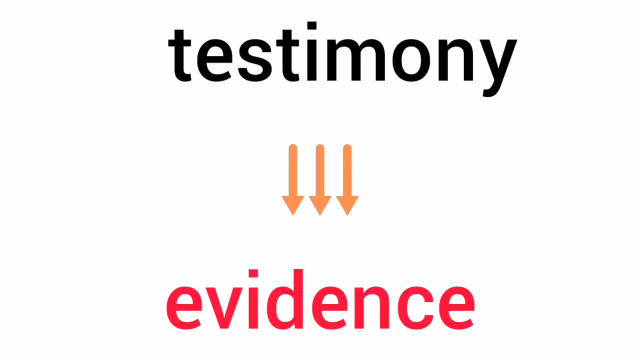 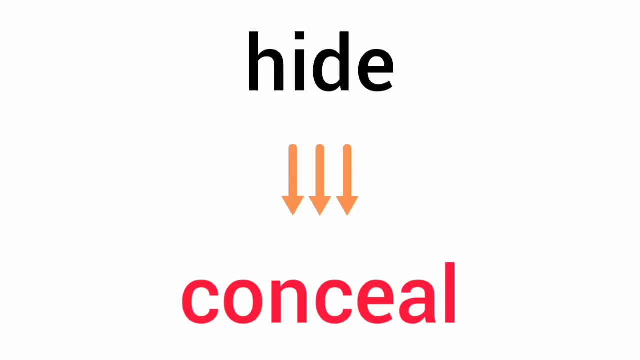 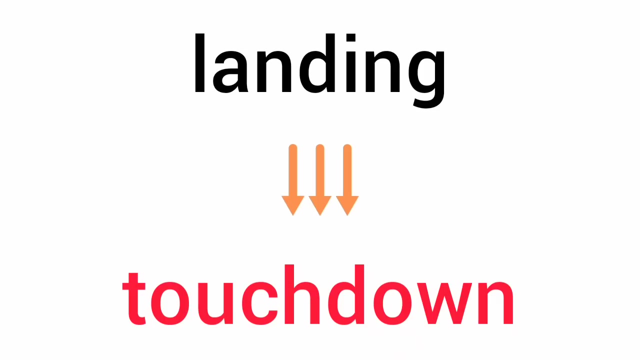 Shiver, mood, temper, mood, temper, rush, hurry, rush, hurry, fair, reasonable, fair, reasonable. testimony evidence. Testimony evidence: Hide, conceal, hide, conceal: landing touchdown, landing touchdown, go, move, go, move, move. 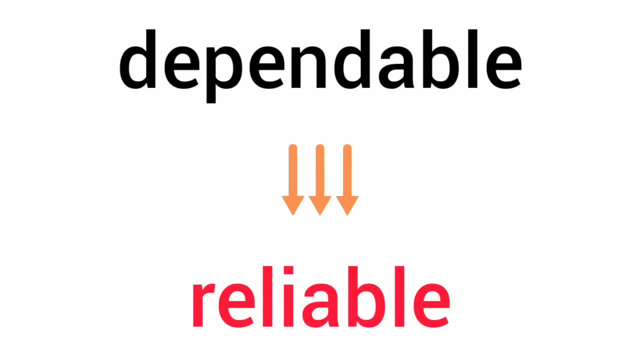 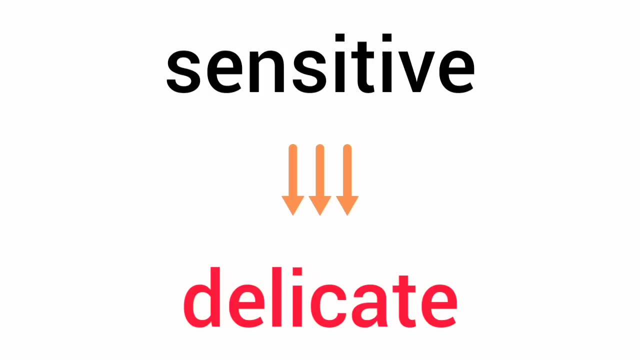 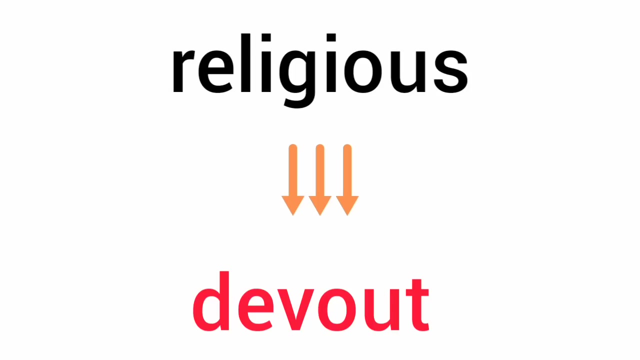 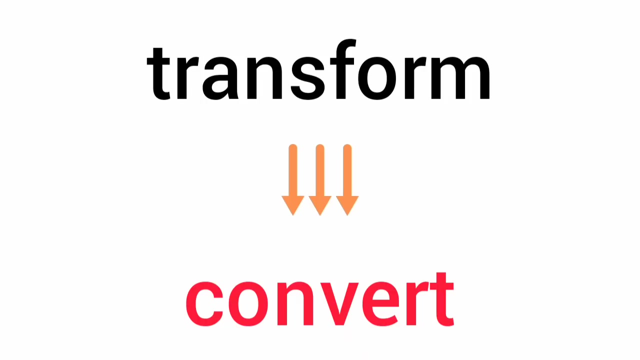 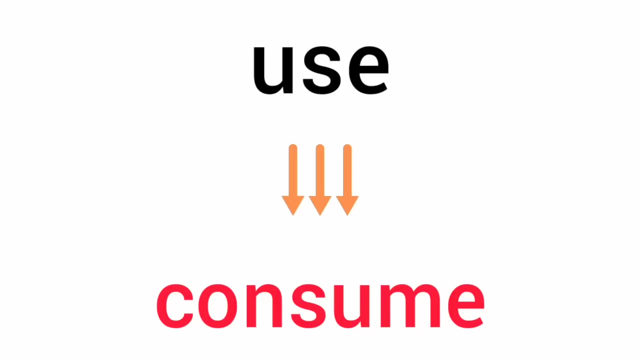 go move: Dependable, reliable, dependable, reliable, sensitive, delicate, sensitive, delegate, Religious devout, religious devout. Transform, transform, transform, transform, transform, transform, Convert, Transform, Convert, Use, Consume, Use, Consume Comment. 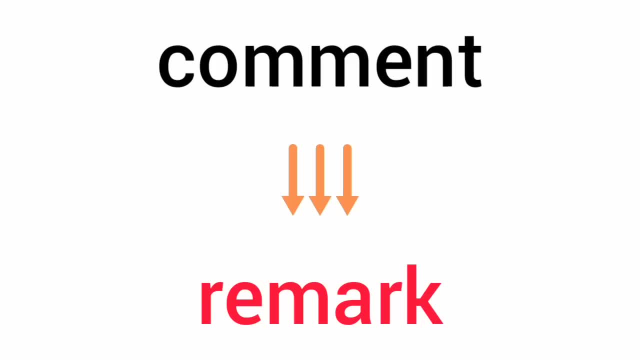 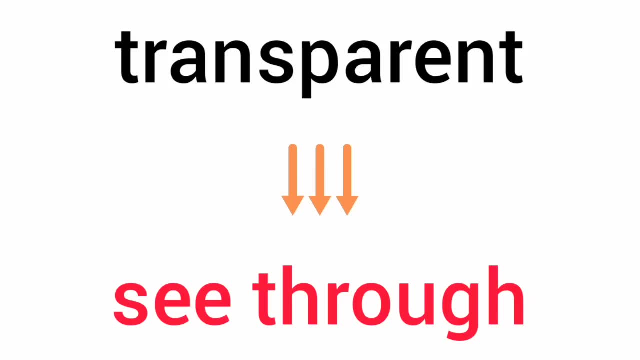 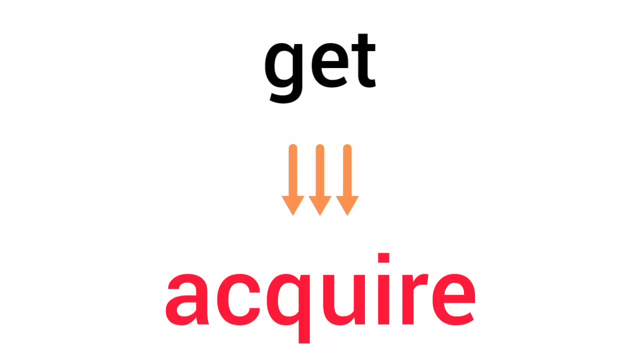 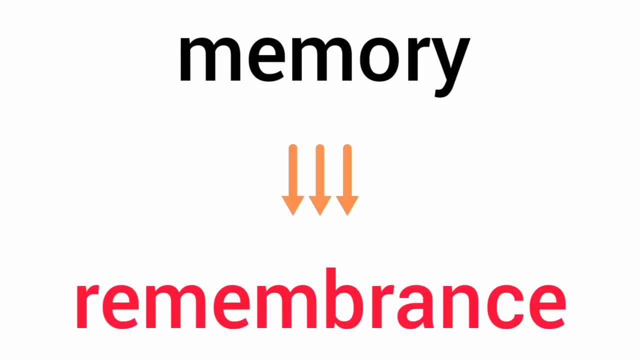 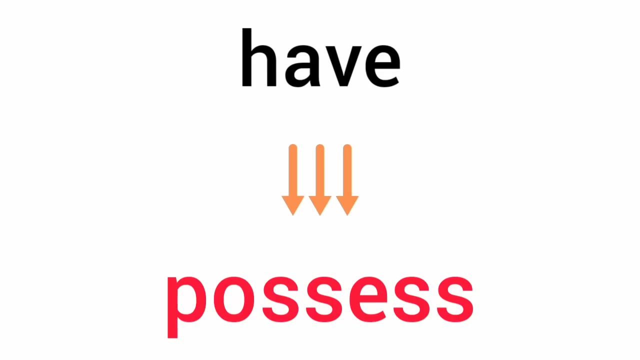 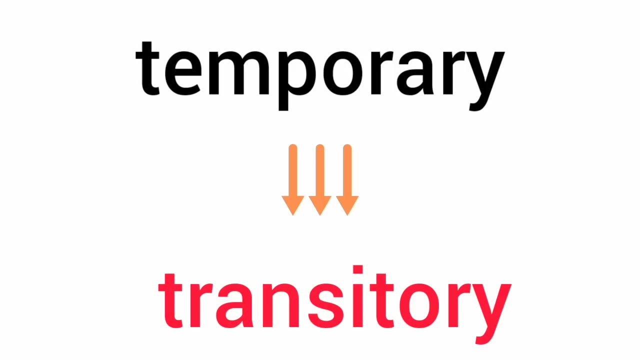 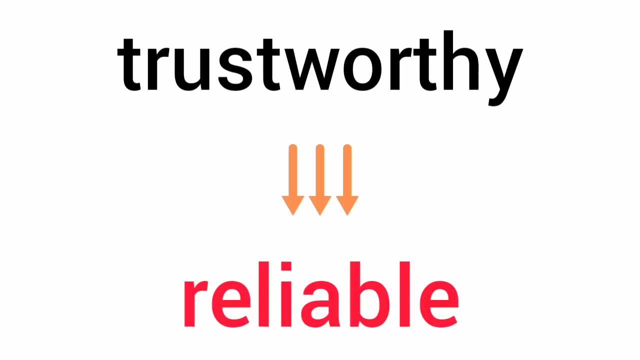 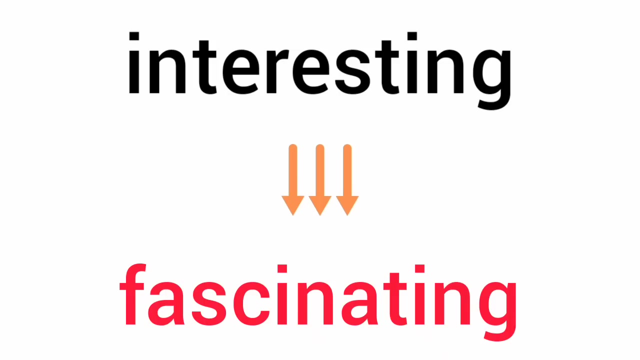 Remark, Comment Remark: Transparent, See-through, Transparent, See-through: Get Acquire, Get Acquire. Memory Remembrance, Memory Remembrance: Have Possess, Have Possess, Have Possess Rest, Remainder Rest, Remainder Temporary Transitory. Temporary Transitory: Trustworthy, Reliable, Trustworthy, Reliable, Trustworthy, Interesting. 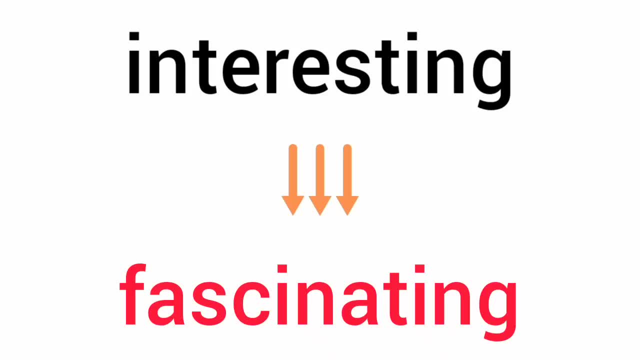 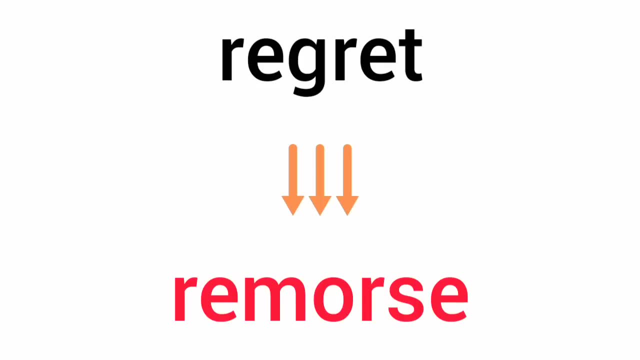 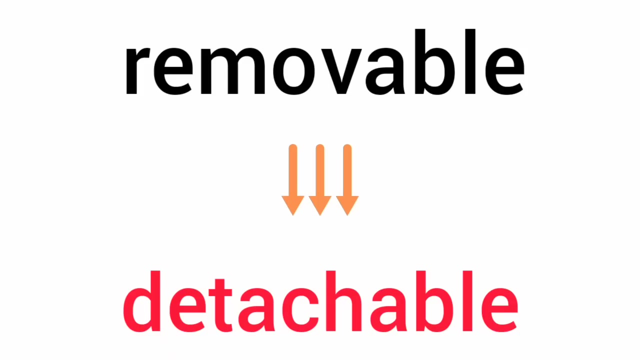 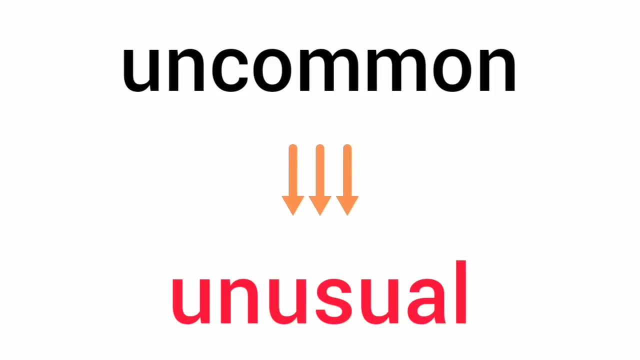 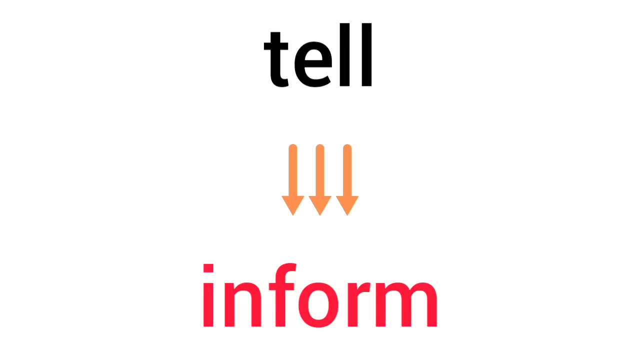 Fascinating, Interesting, Fascinating. Regret, Remorse, Regret, Remorse, Pair, Pair, Dual Pair, Dual, Kind of Slightly, Kind of Slightly Final, Ultimate, Final, Ultimate, Removable, Detachable, Removable, Detachable, Uncommon, Unusual, Uncommon, Unusual, Tell, Inform, Tell, Inform, Resume. 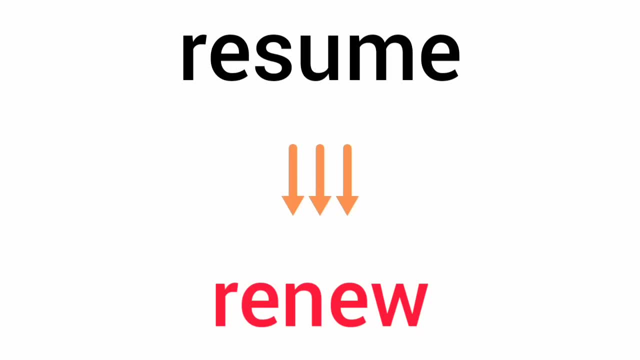 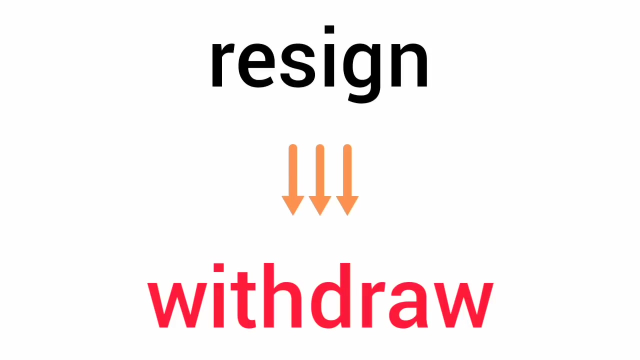 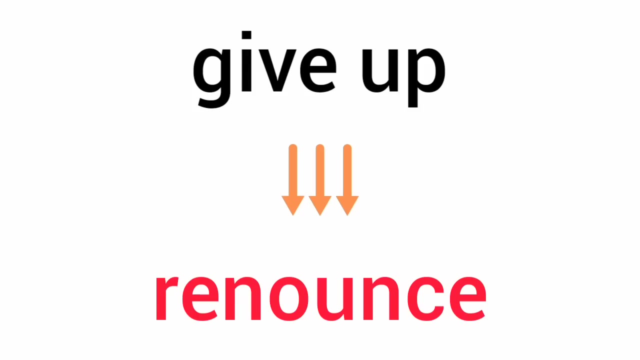 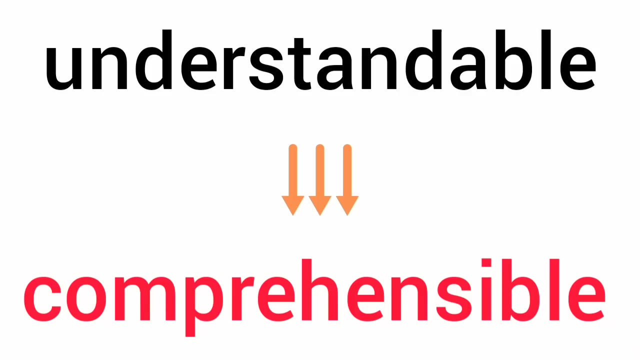 Renew Resume. Renew Roar Uncooked, Roar, Uncooked, Uncooked. Cry, Cry, Sob, Cry, Sob, Cry, Cry, Sob, Sob, Sob, Resign, Resign, Withdraw, Withdraw, Withdraw, Withdraw, Give up, Give up, Renounce, Renounce, Give up, Renounce, Give up. Unstable, Unstable Be Ask. 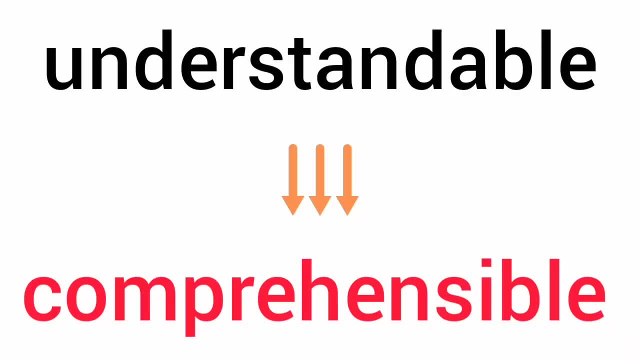 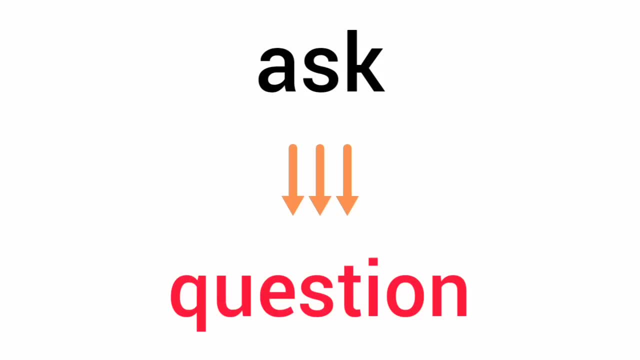 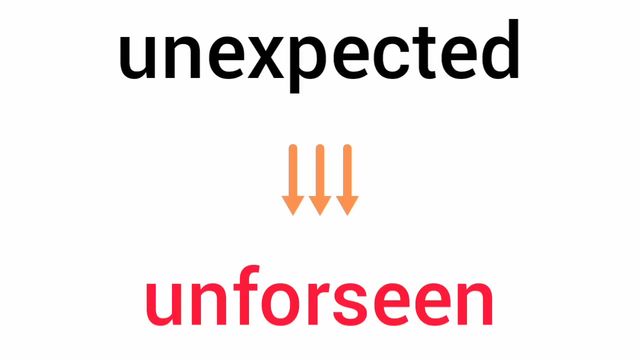 fps Compact Make Demand Unstable. Tell, Ask, Ask Ask. Connect Music Capture Th vari. Ask Question, Ask, Question, Ask, Ask, Ask, Ask. Repligh Question, Respond Reply, Respond Reply. Respond Unني Fri. If Any Reply Respond Unexpected, Unforeseen, Unexpected Unforeseen. 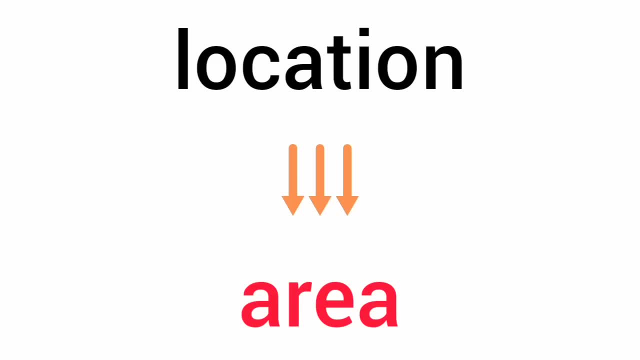 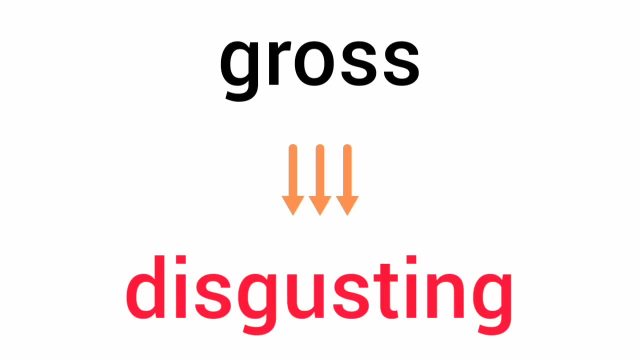 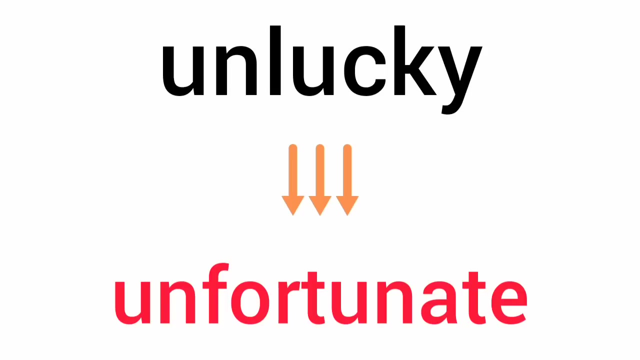 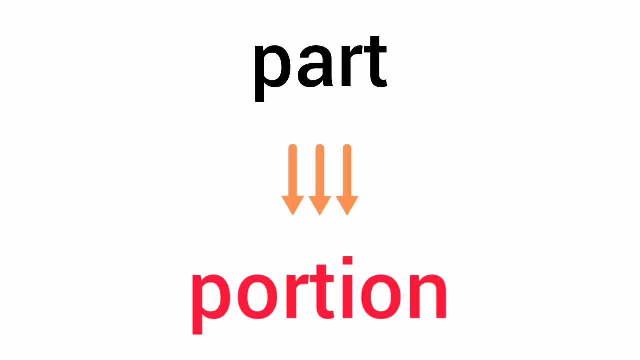 Location, Area. Location Area: Gross, Disgusting, Gross Disgusting, Unlucky, Unfortunate, Unlucky, Unfortunate. Part Portion, Part Portion: Garbage Trash, Garbage Trash. 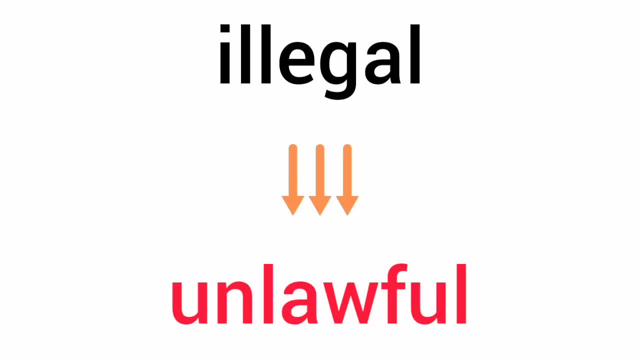 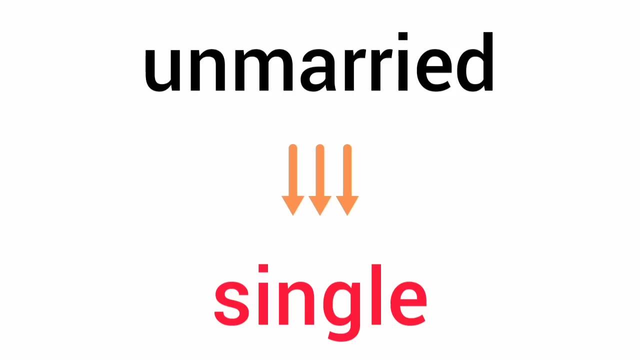 Illegal, Unlawful, Illegal, Unlawful, Rude, Impolite, Rude, Impolite, Unmarried Single, Unmarried, Single Sure, Certain Sure, Certain. Regret, Rude, Regret, Rude. 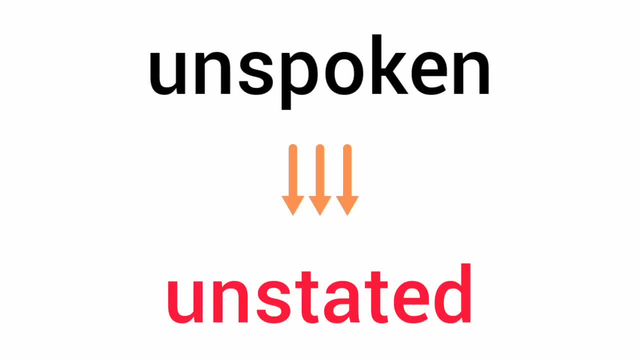 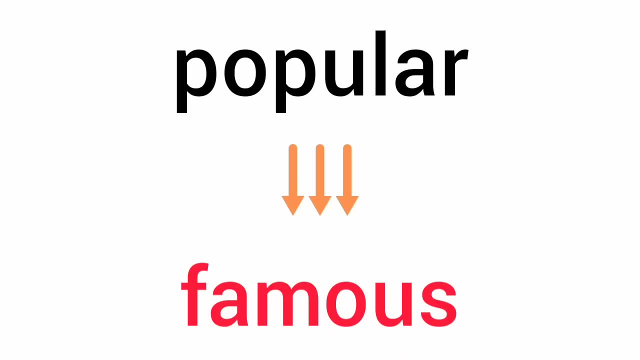 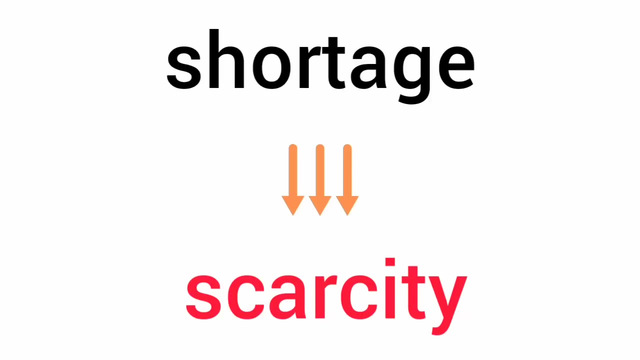 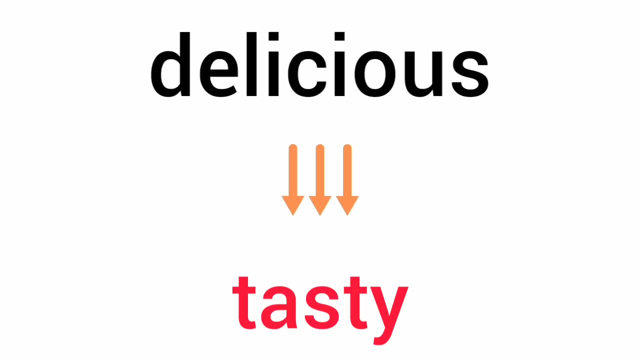 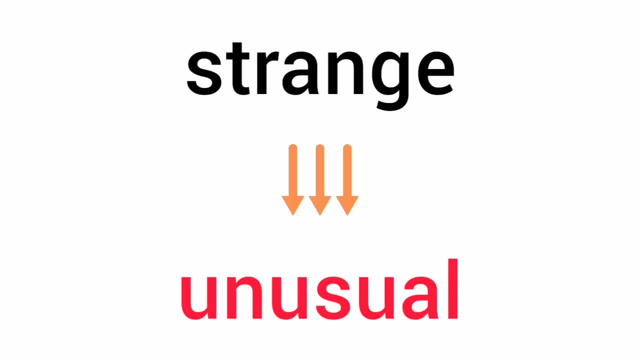 Unspoken, Unstated. Unspoken, Unstated, Popular, Famous, Popular, famous, shortage, scarcity, shortage, scarcity, lie, untrue, lie, untrue. clean, neat, clean, neat, delicious, tasty, delicious tasty, strange, unusual, strange, unusual, playful. 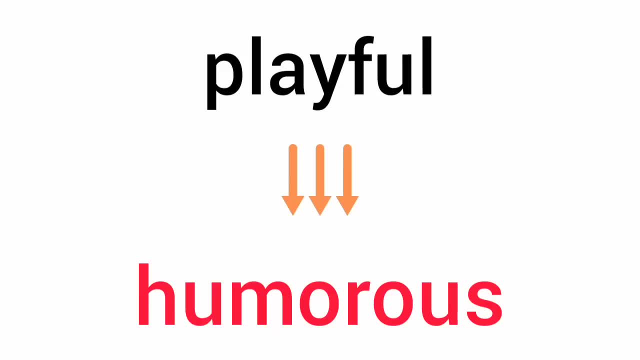 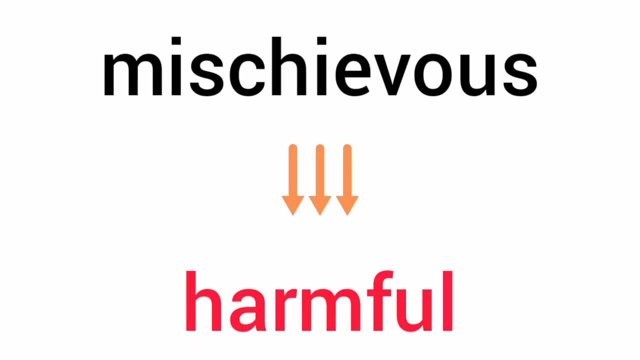 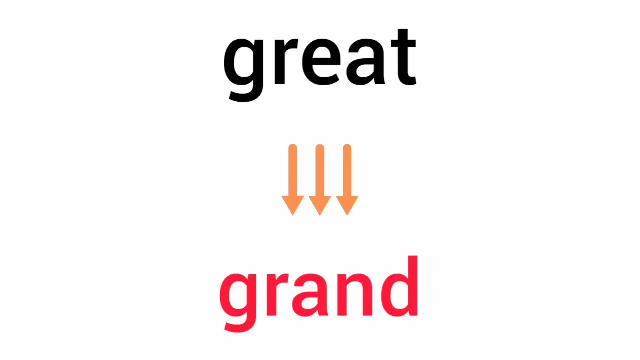 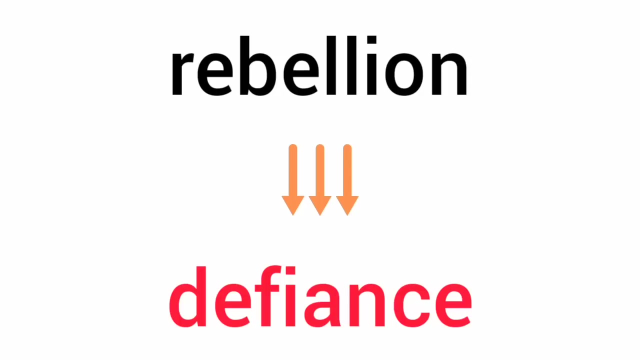 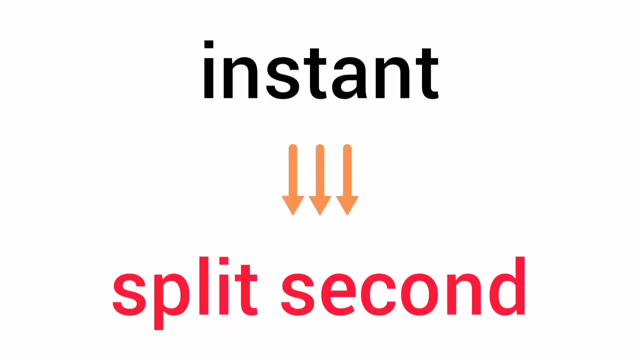 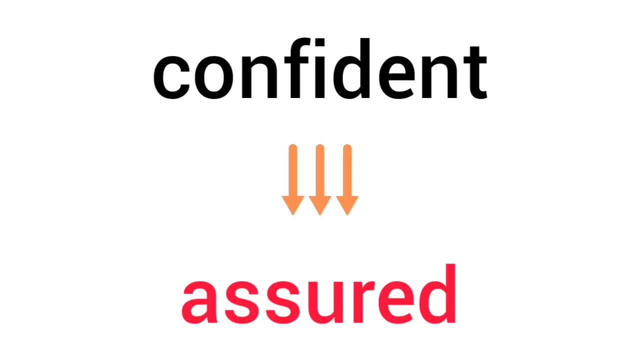 humorous, playful, humorous, mischievous, harmful, mischievous, harmful, great grand, great grand rebellion, defiance, rebellion, defiance, instant, spontaneous, split-second, instant, split-second, confident, assured, confident, assured, unclear, vague. 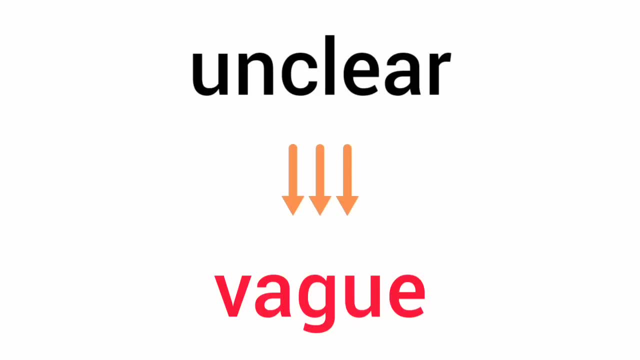 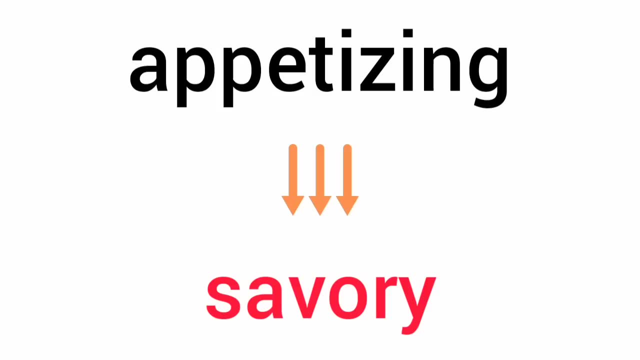 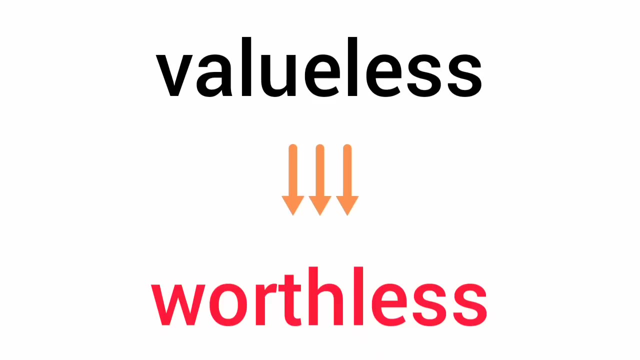 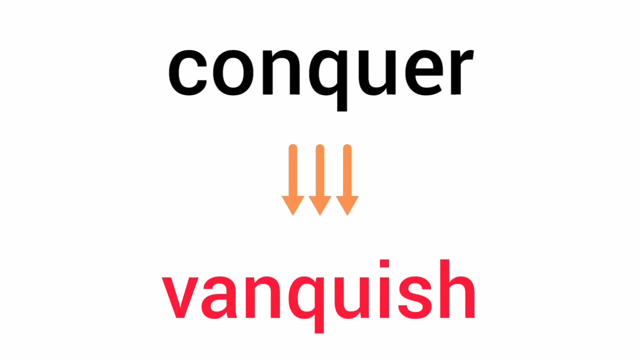 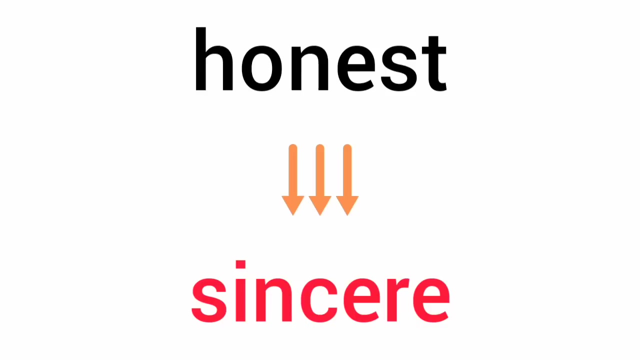 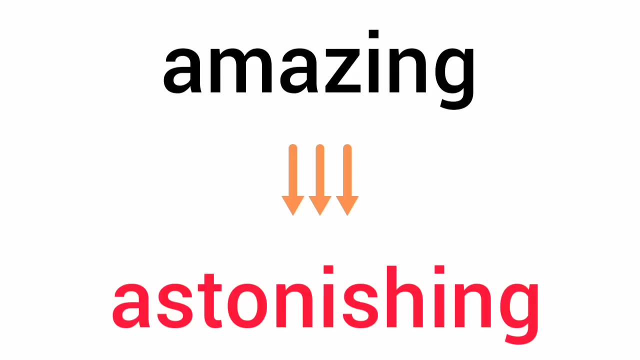 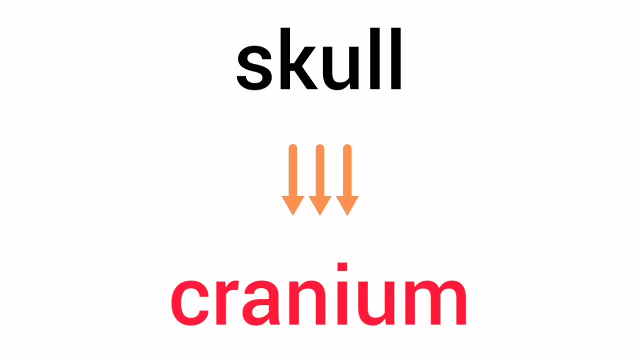 unclear, vague, appetizing, savory, appetizing, savory, valueless, worthless, valueless, worthless. conquer, vanquish, conquer, vanquish. honest, sincere, honest, sincere year. Amazing, Astonishing, Amazing, Astonishing. Skull, Cranium, Skull Cranium, Differ Very. 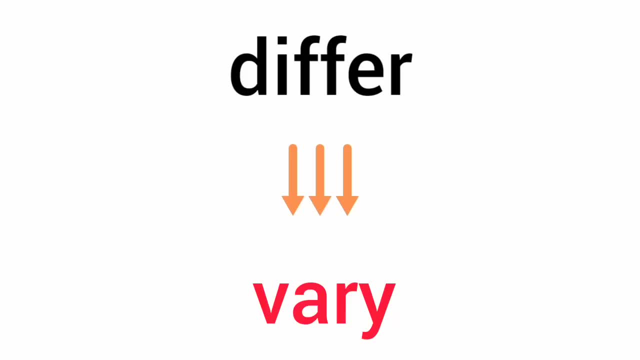 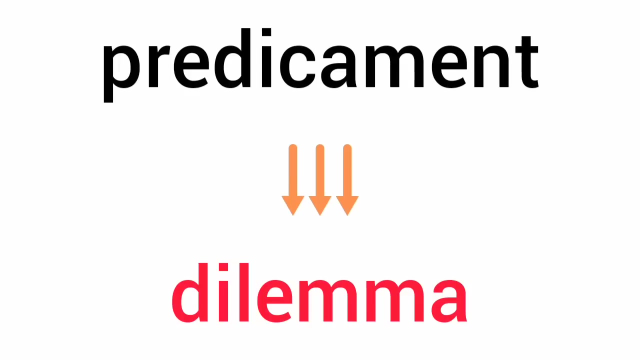 Differ Very: Ugly, Hideous, Ugly, Hideous, Dirty, Soiled, Dirty Soiled, Vast, Huge, Vast, Huge, Trouble, Distress, Trouble, Distress, Predicament, Dilemma, Predicament, Dilemma.